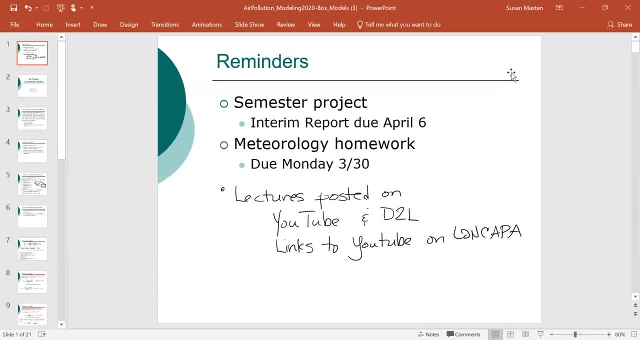 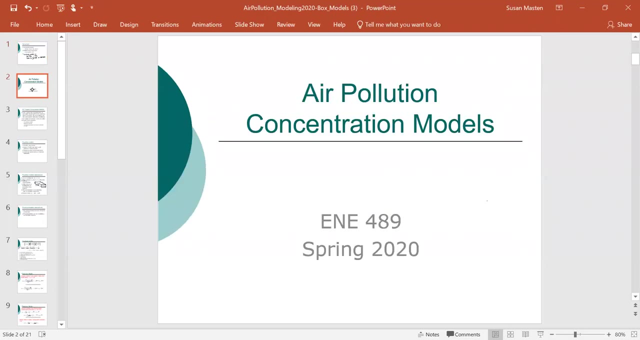 I don't know how much. Okay, I'm Discord, I'll have on D2L, but for now I'm posting both locations and the links to the YouTube videos are online Kappa. So let's look at air pollution concentration model. 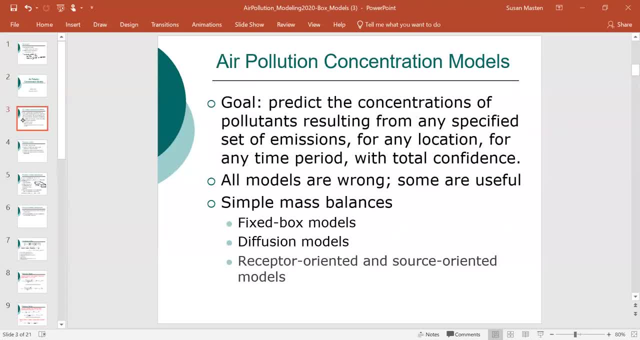 So what we're attempting to do here is what we want to be able to do- is we want to be able to predict the concentrations of high pollutants. So if we have a stack, as we mentioned, we've done, looked at meteorology, So we have this: these pollutants. 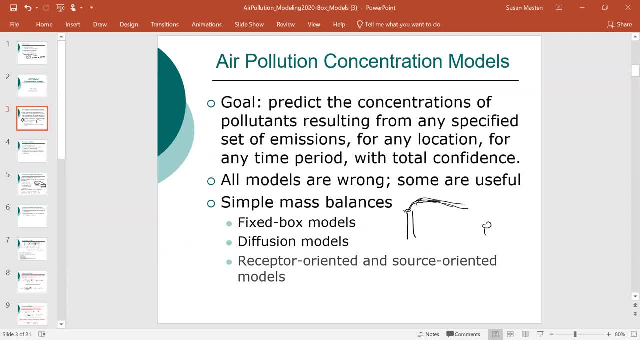 Here's our stack, Here's our person And maybe we have a tree here. We want to be able to determine What impact That pollutant may have on that tree, on that person, etc. So we're looking at predicting concentrations of pollutants. 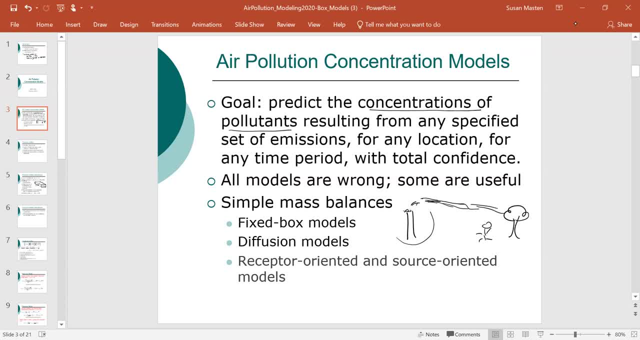 We want to be able to quantify how much emissions. We're also very concerned with the meteorological conditions that dictate how This pollutants will move, And ideally we want to be able to do this with total confidence. So we want, ideally, a perfect model. 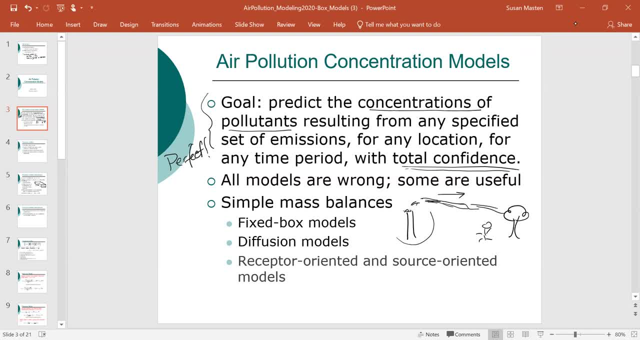 Unfortunately, there are no perfect models. It's one saying that all models are wrong. Some are useful, None of them are perfect And none of them predict exactly Where these pollutants will be in, exactly what these, What their concentrations are. But we still can use these models. 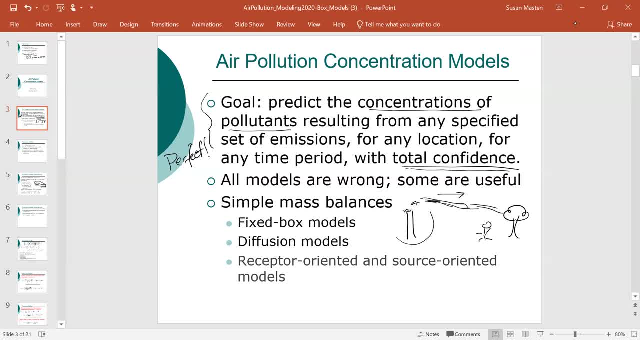 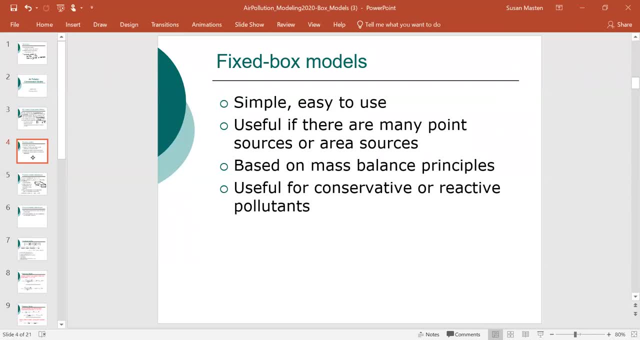 And we'll talk about some of these uses a little bit more. But basically what we're looking at Is We want to be able to predict, for instance, where they initial permitting Application. What might we expect In terms of concentrations downwind? 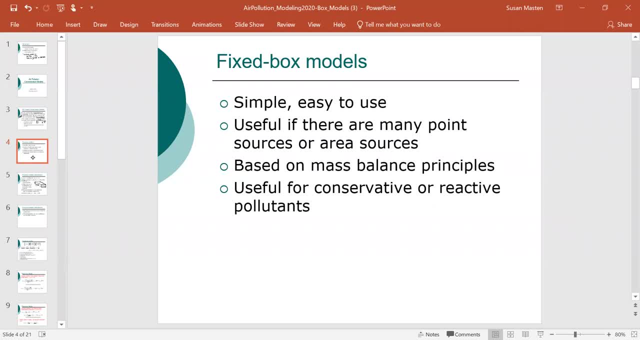 All of these Are Based on mass, Mass balance principles. So, whether we use a Gaussian Model or a FIC- what we refer to as a fixed box model- They're all based on mass balance. The fixed box models are relatively simple, relatively easy to use. 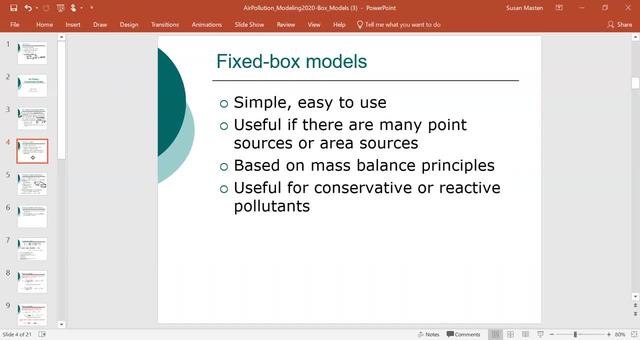 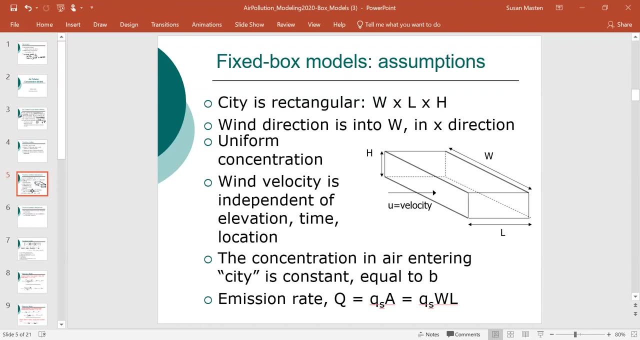 We can use those if we have multiple Point sources, We can use them if we have area sources, And we can also use them if we have both conservative or reactive pollutants. Now, the approach that we're going to use here: This is essentially the same approach that we used with indoor air pollution. 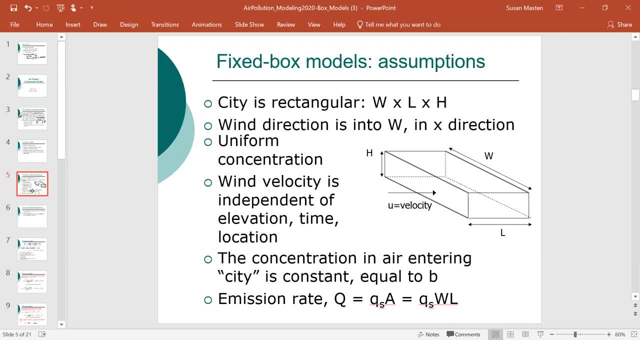 It's a little bit different Aspects in terms of the notation that is conventionally used. So, for instance, with Indoor air Pollution, We looked, we used The air changes per hour. Typically we don't use air changes per hour. 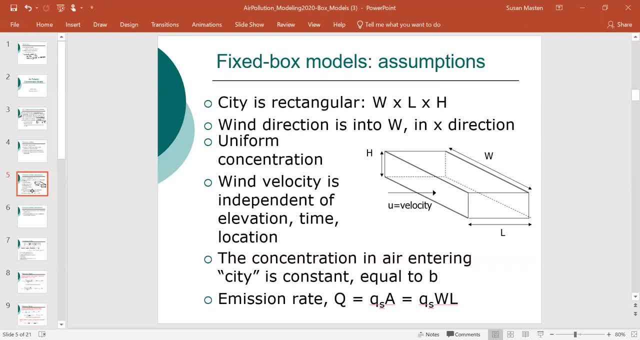 For these box models, But instead we will Use the velocity, because what do we typically measure? You look online. Okay, I want to look at what the weather is. I'm going to look up what the wind speed is. I'm going to look at what the temperature is. 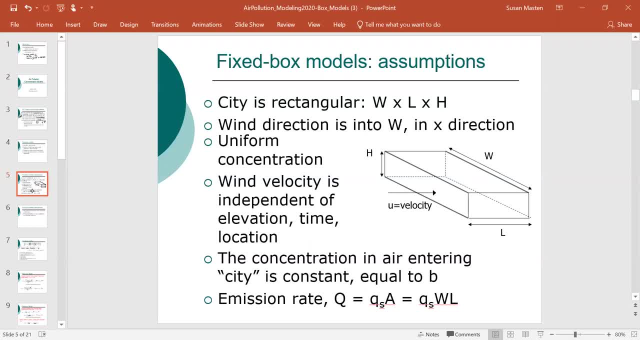 I'm going to look at what the temperature is. I'm going to look at what the wind speed is. Okay, So What these models do Is we're going to assume That we have some sort of a rectangular Box This height here. 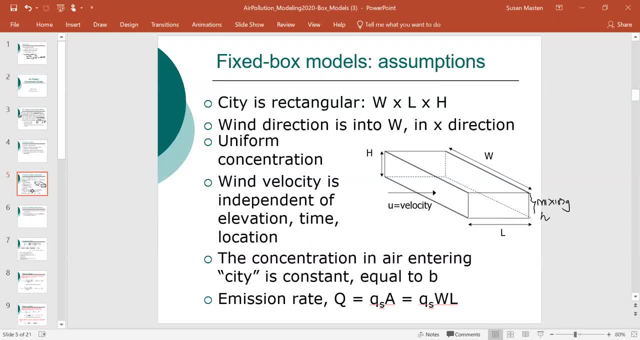 Is our mixing height. So we've talked about the mixing height and showed how to determine the mixing height, So that H is our mixing height. We're looking at wind Entering Along the width. So this is her with here. You can see it along here. 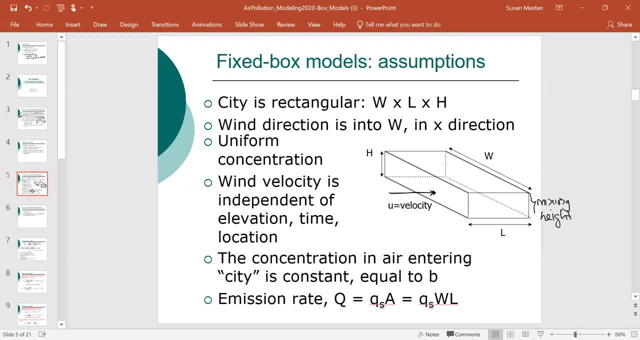 And the wind enters along this Face Of our box, We'll assume that we have uniform concentration. So we're going to assume That. the assume that we have a well-mixed system, if this would allow me to do this. okay, so we have a well-mixed system, so the concentration at any point in the box is: 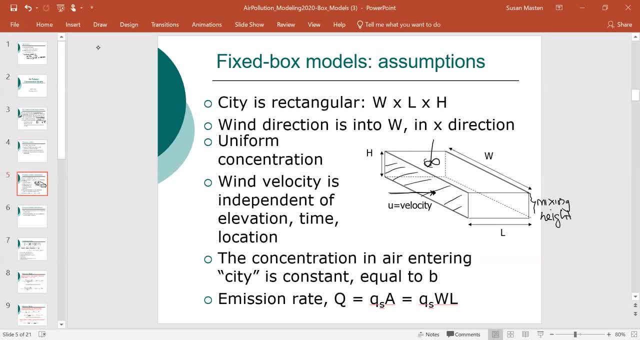 the same also as we've discussed before. if that is the case, then the concentration in my box is the same as the concentration leaving my box network, also assuming that this wind speed is independent of elevation, it's constant and it doesn't depend on the location. so I put這些 之。. 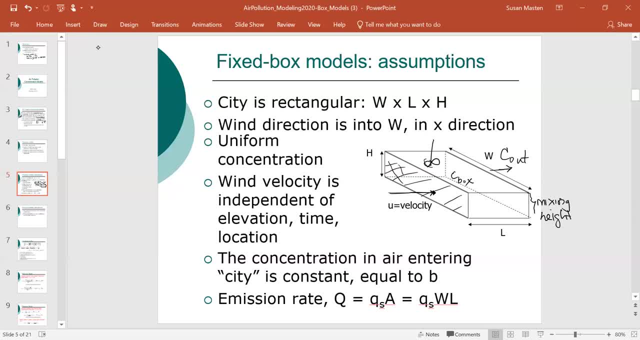 If I were to measure the wind speed anywhere along this space, it would be the same. We know that's an approximation. however, that's the assumption we're going to make. We will also assume and we'll use the term B we used before. we used Cn or C ambient. 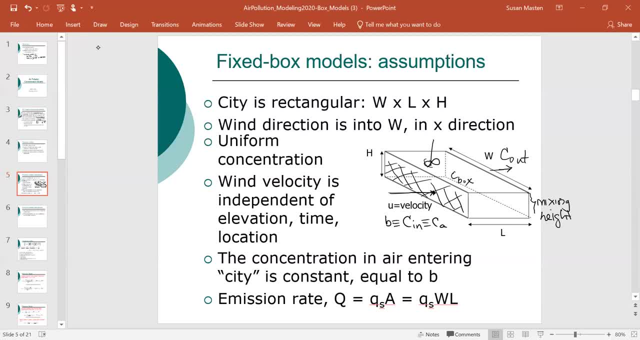 what we used when we talked about indoor air quality. The notation here that's used is often B, So that's the concentration entering this space. Okay, We also talked about- we talked about a source term before, so S and notation that's typically. 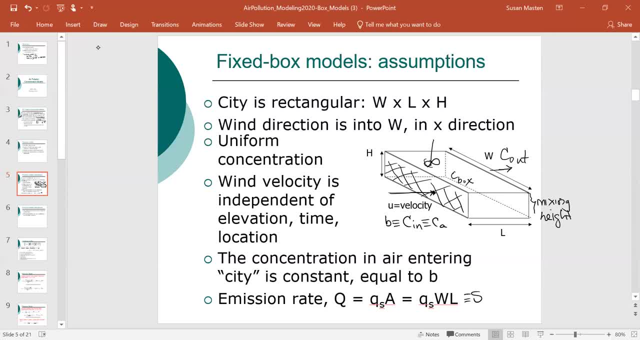 used here is Q and we have a Q that is both a mass per time, and we have Q sub S, that is, mass per area per time. Okay, And the area that we're going to use is the width and the length. So we're looking there, I'm going to change color. 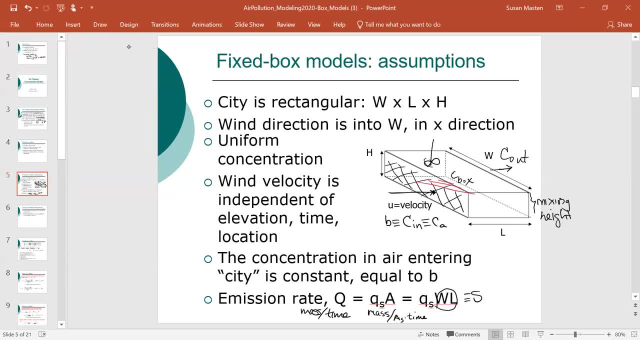 So, there, what we're looking at is we're looking at this area here, so we're looking at the base then of the model. So this corresponds to the red area, Okay, Okay, So this is the red hatched area. On the other hand, going back here, this U we're looking at the black hashed area along. 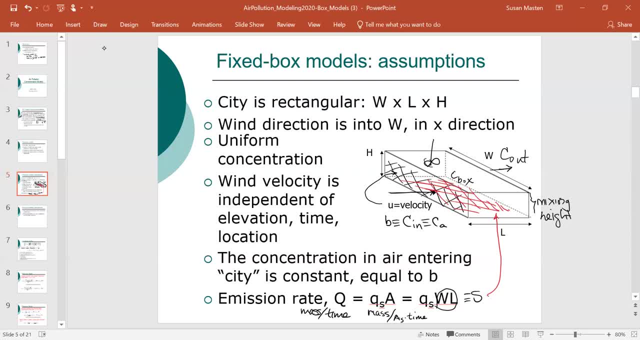 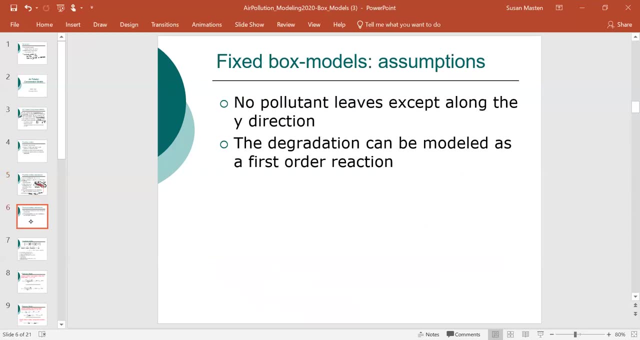 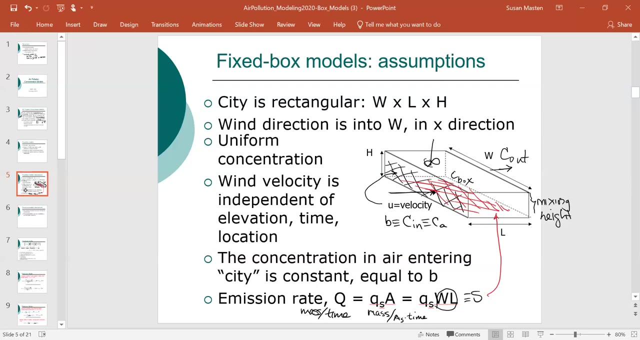 that face. Does that make sense? Because this is important, So we can move forward, Okay, Okay. The other thing we are going to assume is: then let's go back to this model here, And now let's we'll pick another color here. 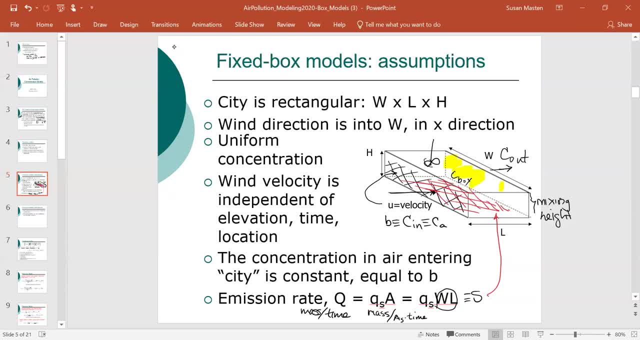 We're going to look at this face right here. All of the pollutant that leaves is going to leave from that face. So there's no pollutant leaving out of the top, There's no pollutant leaving out of the sides. It simply moves in from the one face here and moves out to the other. 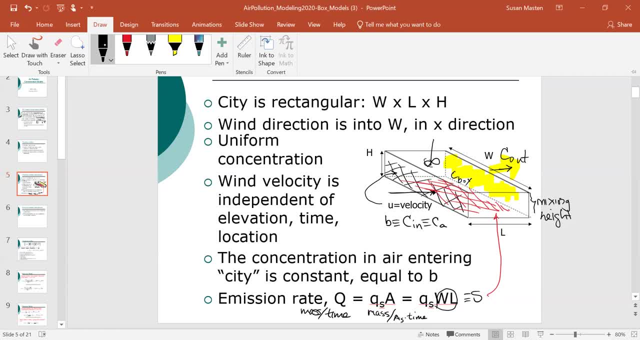 Okay, And then the last thing we will assume is that we can use first order kinetics. So again we just have. the change in concentration with respect to time is equal to 1.. Okay, Okay, Okay, Okay, Okay, Okay. 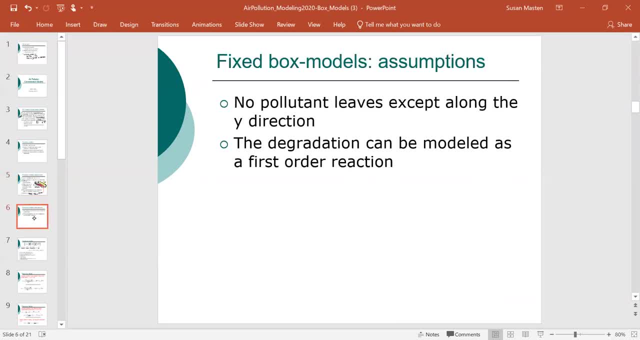 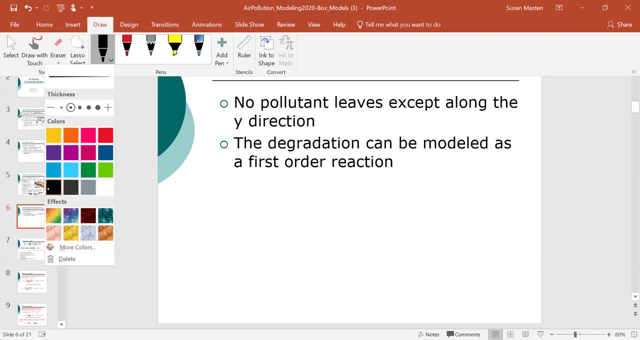 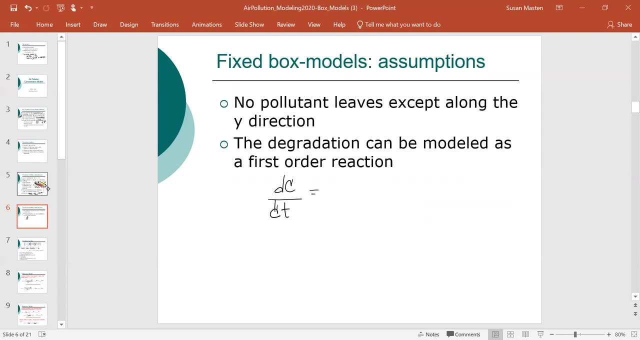 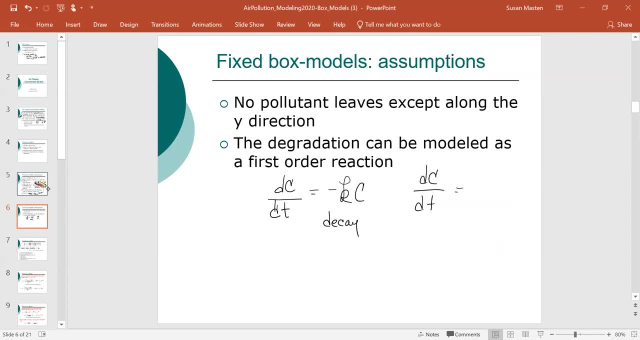 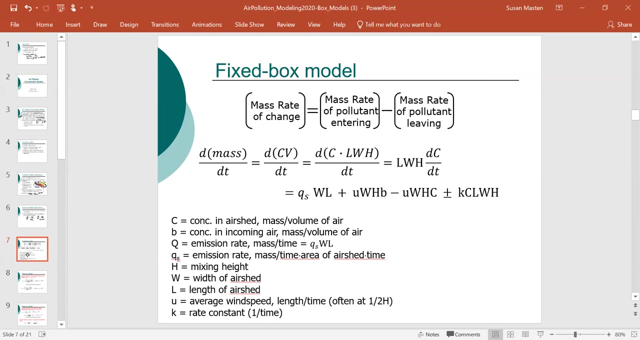 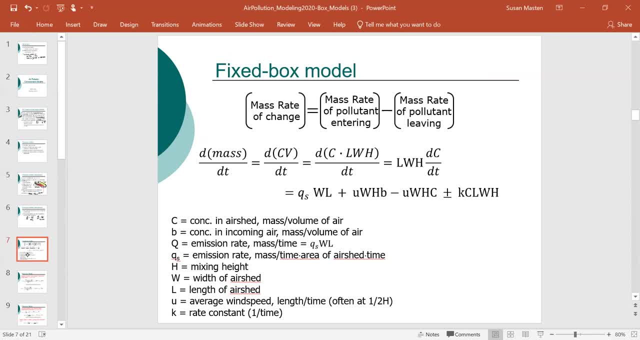 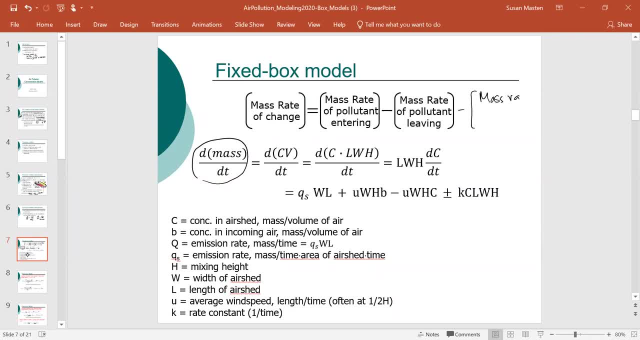 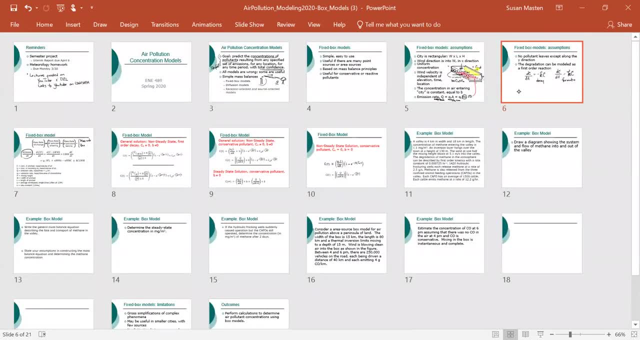 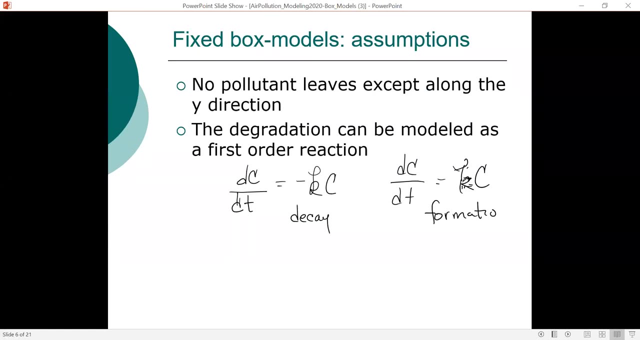 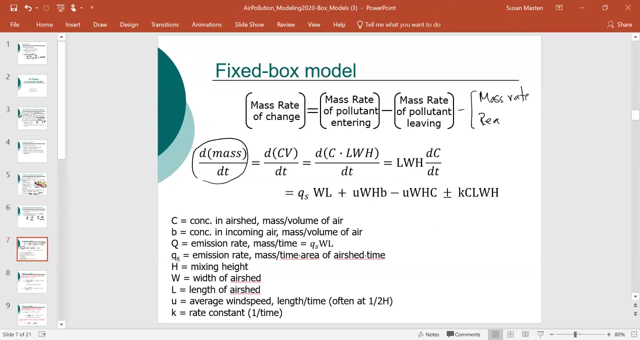 in here. then we have the mass grade reacting- sorry about that- the mass rate reacting. so what are we assuming? so our mass is equal. so we, so our mass is equal. if mass is equal to concentration times volume, same as previously in the semester. this volume is equal to our length times our width, times the height, and if this is constant. 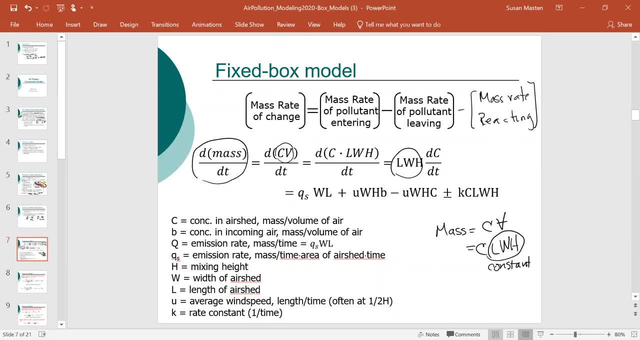 then i can remove that. it's now a constant, it's outside of my differential, and what i have is: i then have my length, width, height, dc. dt is equal to. this is a source term: the: what is entering through the face, what's leaving out the up. 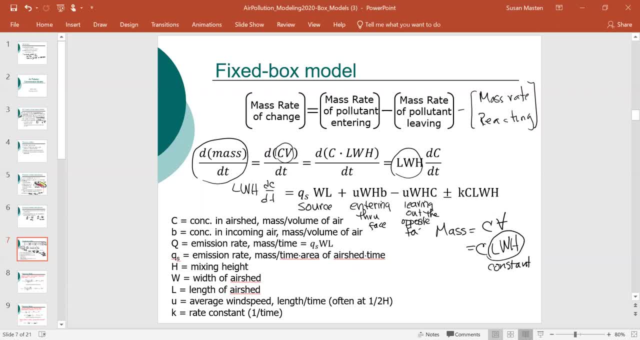 opposite face and what is reacting. so here, if it is reacting and we're losing chemical, then it's going to be negative, so that's loss, and if we have formation, then it's positive. so we can actually write this expression with either formation or loss of the, the pollutant i'm looking at. 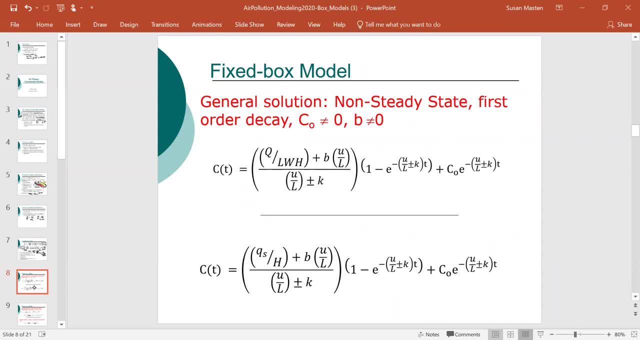 so what i've done is i've developed a series of equations for you, so we have both the. i'll give you both the non-steady and the steady state. so notice here: okay, this is the non-steady state form with first order decay. note here: 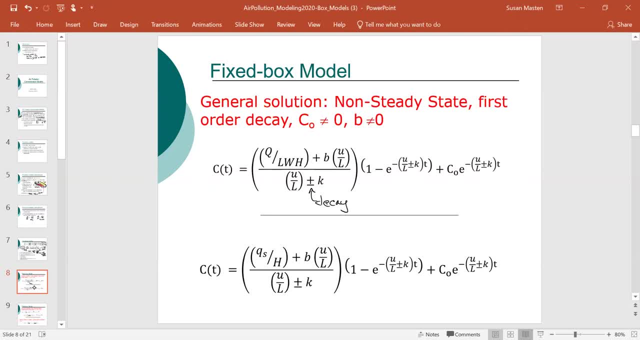 if you have decay, then this term is actually positive. if you have formation, then it's negative, and that's because the terms actually switch. think of this: if it's both decay, then these, you want, these terms need to add together and that's the same in here. okay, so with all of these terms here, 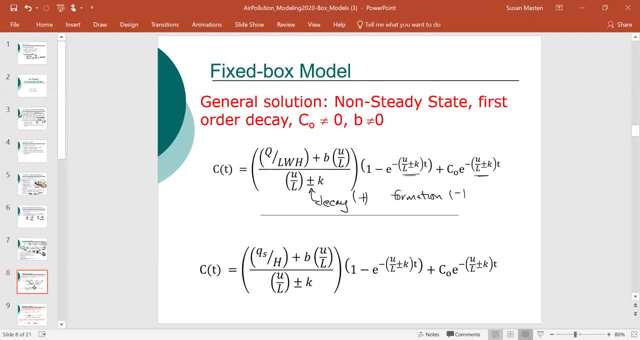 it's essentially the same equation. if you go back and you look at the equations that we used for indoor air quality, it is essentially the same equation. okay, notation was different, but it's essentially the same equation. so, for instance, this u over l term, and why does this not write sometimes? 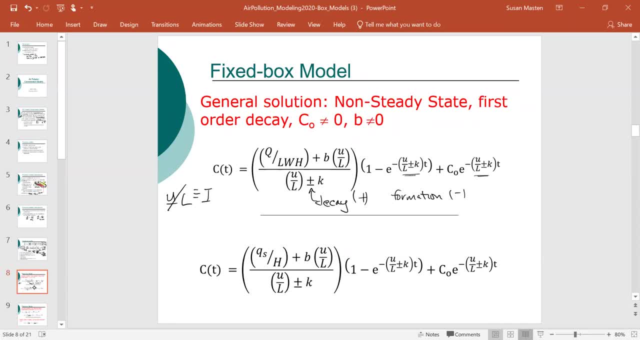 this was equivalent to i when we looked at indoor air. so if you go back and you look at these, these equations are essentially the same- notation is different, but it's essentially the same equation- and then this term here corresponds to that initial state. i've written the equation both in terms of q and in terms of a specific q, so remember this q sub s. 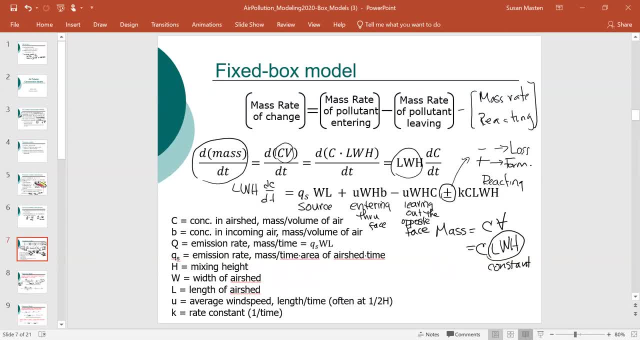 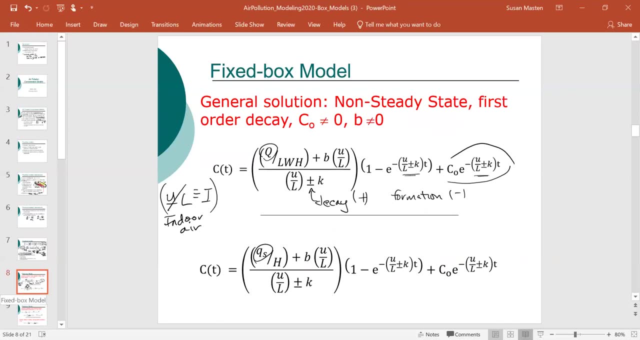 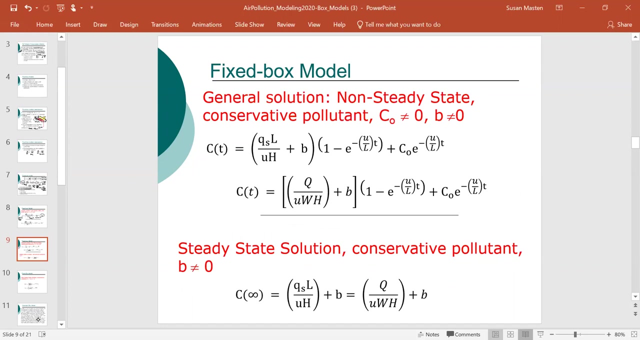 go back here. okay, so q sub s and q sub a are related here, okay, so just so i've done this, we've divided it by two. so the one I've done is I've given you both sets of equations. this is just the non-steady-state equation. 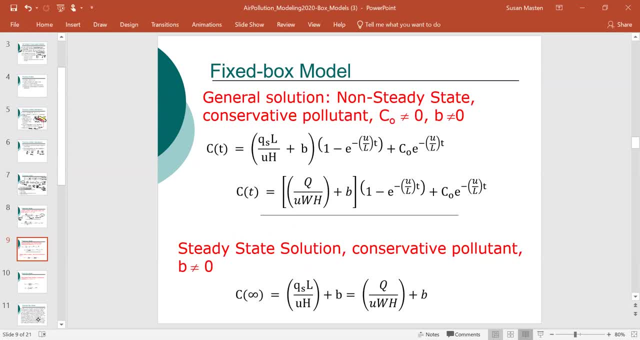 for a conservative. so notice there's no q in this and there's sorry- there's no k, so in this case k is equal to zero, so the k term drops out. this initial term simplifies and, and we have this equation If we have a steady state solution. 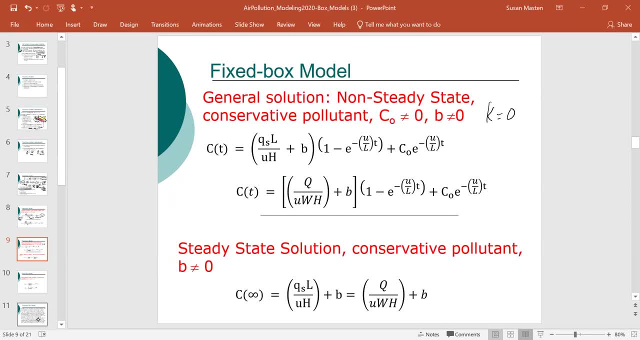 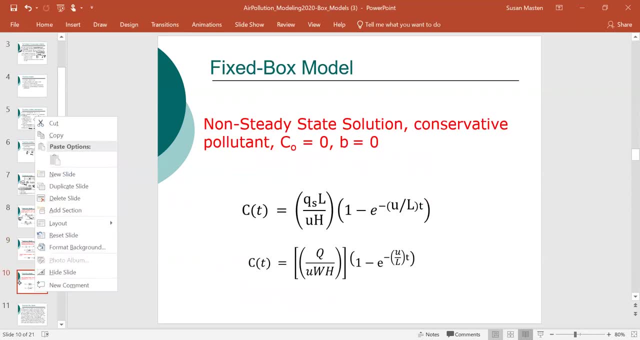 then all the exponential terms drop out and we have a much simpler solution here. And finally, in this case the initial concentration is zero. There's no contaminant flowing into the cell. So we have this equation. So what we're gonna do today? 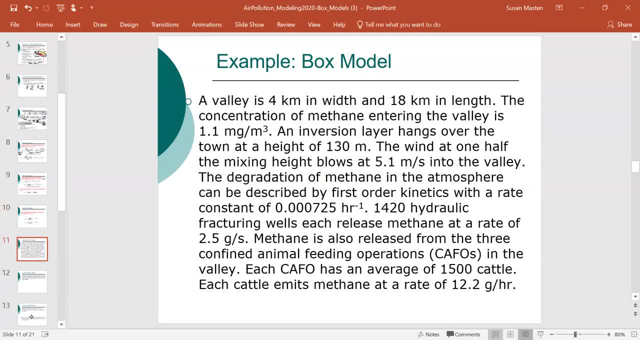 is, we're gonna spend some time mostly doing some problems and looking at how do we approach these problems. So what I'm gonna ask you to do, where you are, is start to write down some of this information. okay, It'll make it easier and I think it'll help. 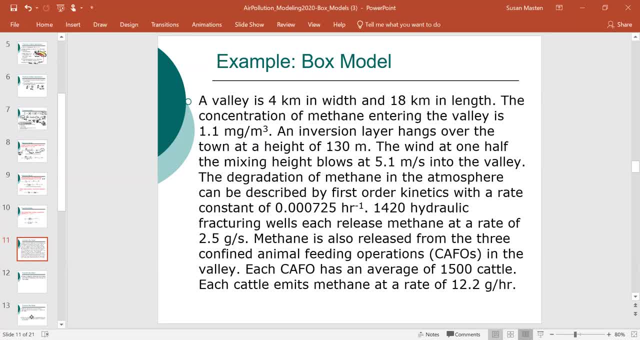 when you're trying to follow through on the computational homework problems. So what do we have? We have a valley, and I'm gonna switch. So we have a valley that is four kilometers in width, 18 kilometers in length, and we have a concentration entering the valley. 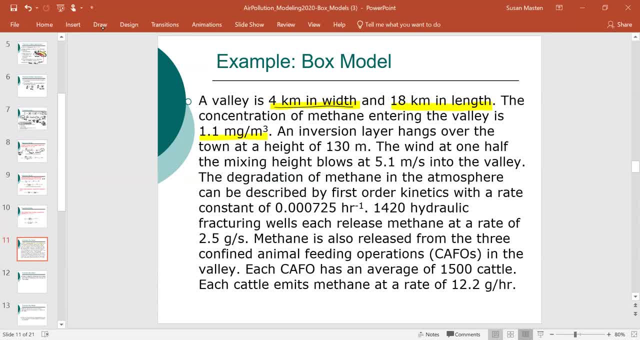 of 1.1 milligram per cubic meter. We have an inversion line and we have an inversion line, We have an inversion layer hanging over the town. So we have a height of 130 meters and we have wind at one half the mixing height. 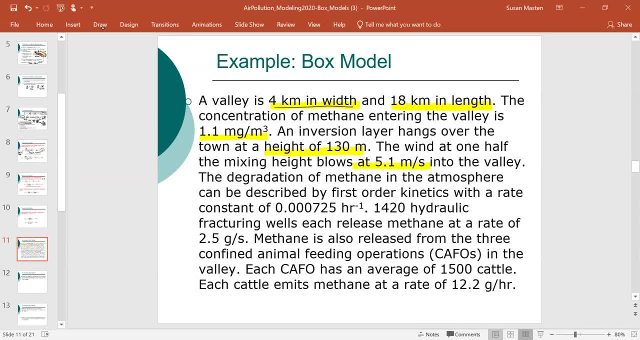 blowing at 1.5 meters per second. So that's the velocity we'll use. The degradation of methane in the atmosphere can be described by first order kinetics, and we have a rate constant of 7.25, and we have a rate constant of 7.25,. 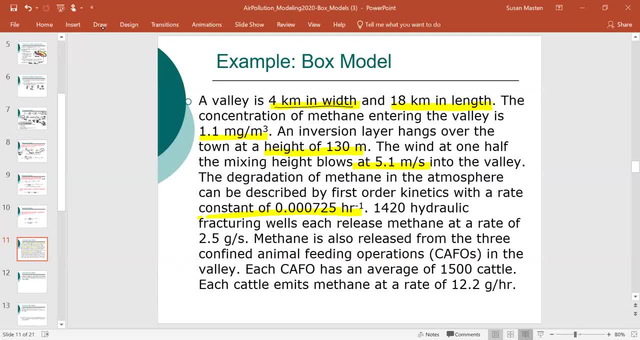 and we have a rate constant of 7.25, times 10 to the minus four inverse hours. And this is an area where we have a significant amount of hydraulic fracturing of fracking wells. We have 1,420 of them. Parts of Pennsylvania would look like this: 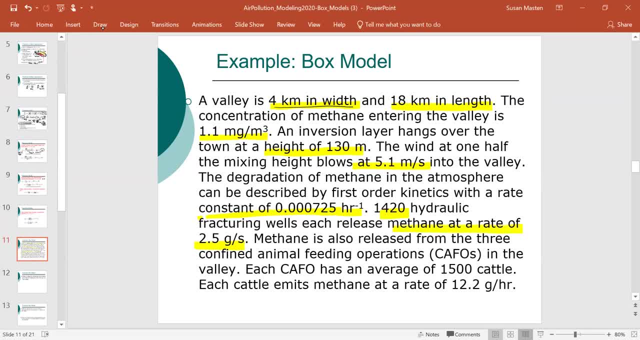 and each of them are emitting methane at a rate of 2.5 grams per second. We also have some confined feeding operations, and each CAFO has an average of 1,500 cattle, and each cattle is emitting methane at a rate of 12.2 grams per hour. 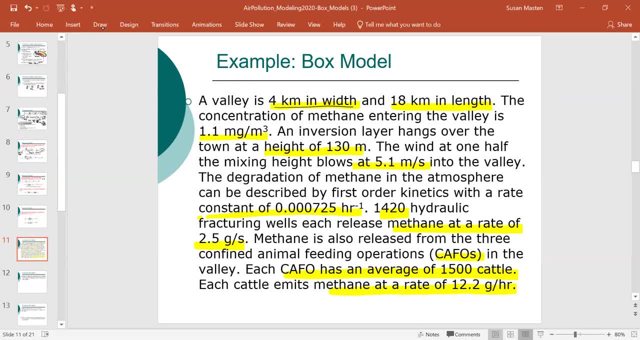 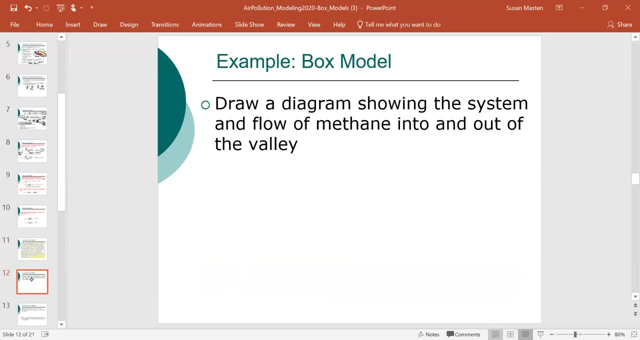 So all that is actually pretty consistent. that's typical emission rates both for a fracking well and for a cow, And we always do that with the most commercial animals, especially unleash animals. But I started to think about that for a second and that was also the case in this area. 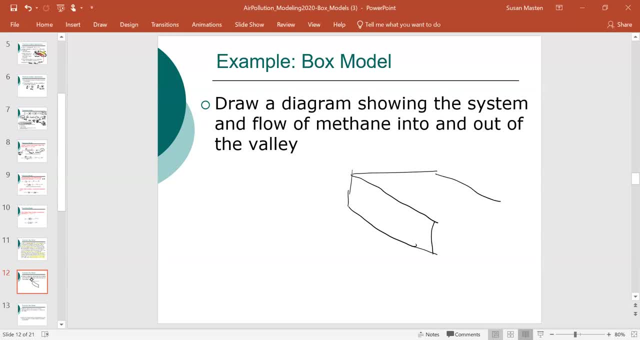 About 10 at first, and then I got in contact with- I'm sorry and I'm thinking about it again- the other one. so here's my box. my width is always in the perpendicular to the wind direction, so here's my wind. we said it was 5.1 meters per second. okay, the length, so the wind. 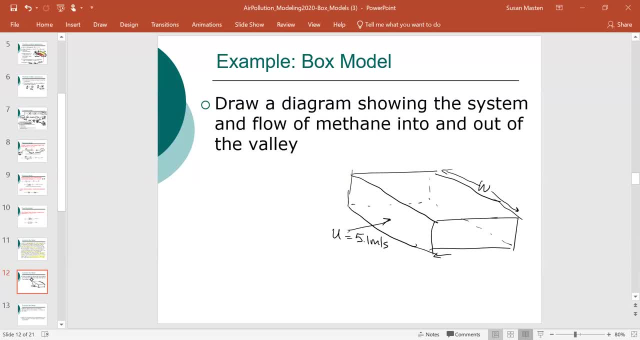 blows along that length and that is 18 kilometers. this is 4 kilometers. the height is 130 meters. we have a concentration of methane entering the cell at 1.1 milligram per cubic meter. you don't know what C out is and we have several fracking wells. 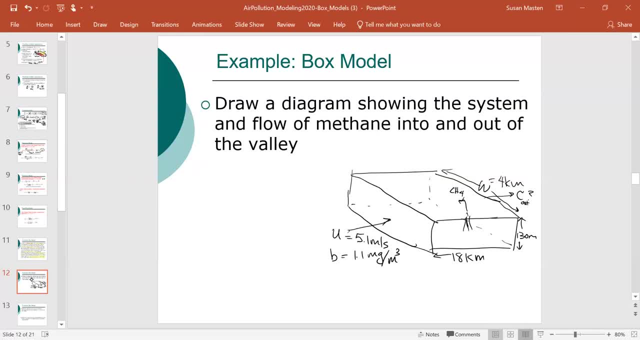 there's new fracking- well, there's new fracking, well, but that's only the first one that we hit are emitting methane, and I'm not very good at drawing cows. here's my cow, there's a towel and we have lots of cows, so we have several forms and that cow is. 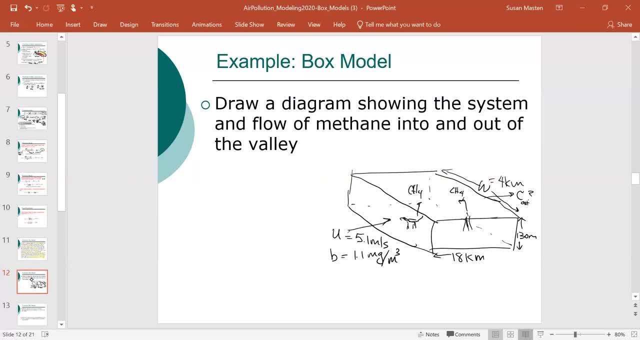 also emitting methane and we can draw- and I'm going to change the color so we can draw our system boundary. so we're looking at methane in, we're looking at methane out of the cell and this would be our cell. we are also must. just we have 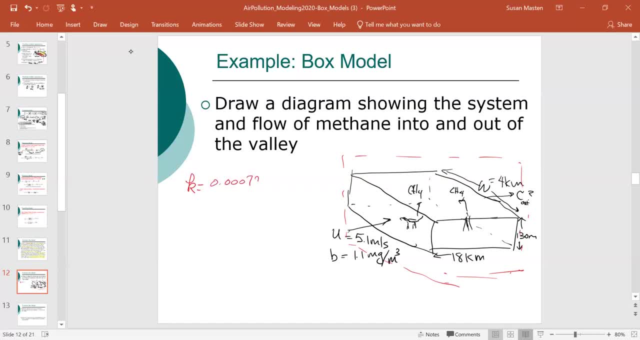 K equals two point zero, zero, zero, seven, two, five in in inverse hours, and that is 2.014. we need other units to be consistent. that's 10 to the minus 2.0 times 10 to the minus 7 inverse seconds. S well is 1420 wells each emitting 2.5 grams per second. so we 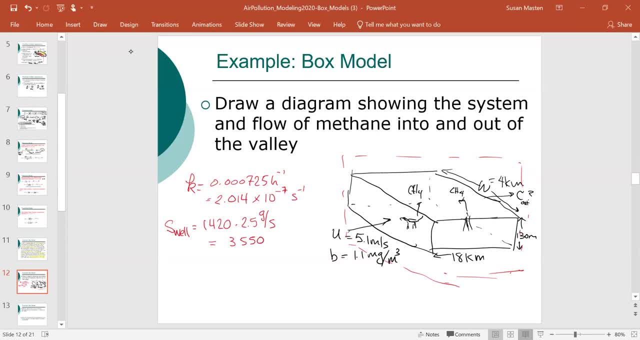 have three thousand five hundred and fifty grams per second being being admitted and from the CAFO's. we have three CAFOs. each has fifteen hundred cows- 12.2 grams per hour and 60 minutes for our 60 seconds per minute And that is 15.25 grams per second. 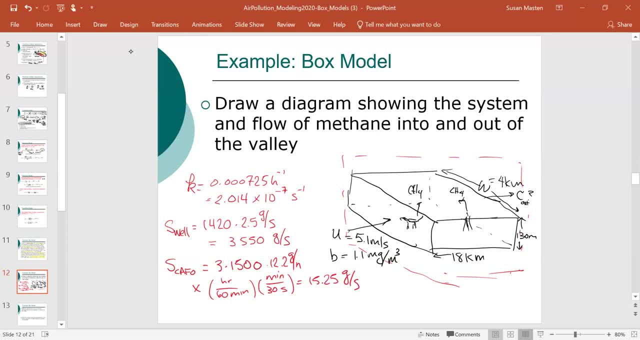 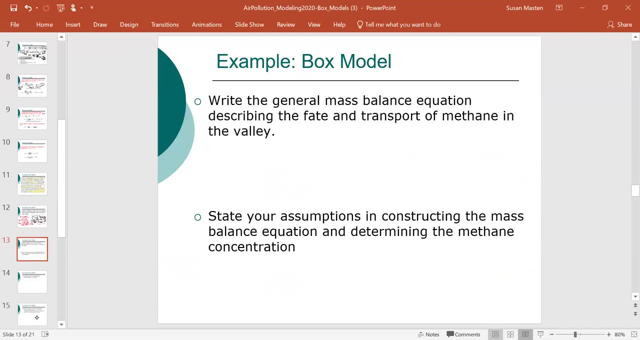 So we have about 15 grams per second from all of the CAFOs and about 3.5 kilograms per second from the fracking wells. So the next thing we wanna do is develop a general mass balance. So what I'm looking for when I ask you to do that. 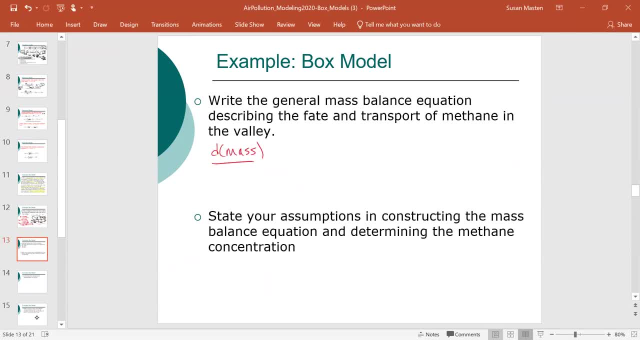 really is thinking about what. I gotta switch back there. What are our source terms? So we have the mass rate in from through the wall or the face of the cell. we have our mass rate from the CAFOs. We have our mass rate from the wells. 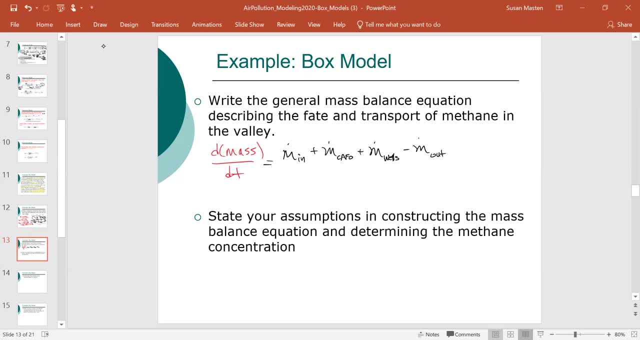 We have our mass out through the opposite face and we have the mass out in a reaction And we can write this: Well, if we assume the volume equals a constant, so I'm just gonna write that down because that's one assumption we can make. 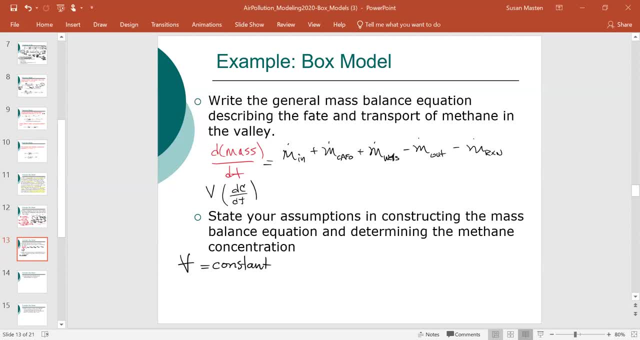 And then this becomes volume DC- DT. And then the mass in is my wind speed times, my concentration times, my width times, my height, plus the mass rate of the CAFO. And then this becomes volume DC- DT. And then the mass in is my wind speed times, my concentration times, my width times, my height, plus the mass rate of the CAFO. 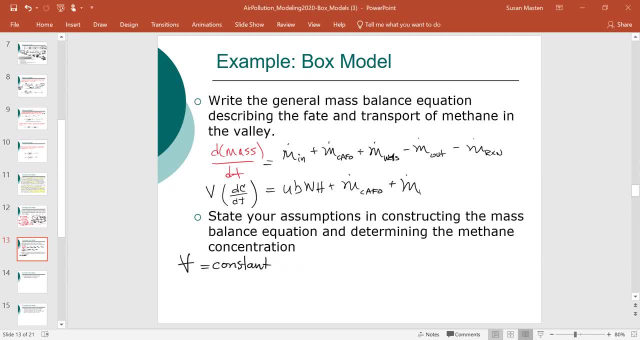 And then this becomes volume, DC, DT, And then the mass in is my wind speed times, my concentration times, my height, plus the mass rate of the CAFO that I calculated, plus the mass rate of the wells, minus U, because we're gonna assume the wind speed leaving. 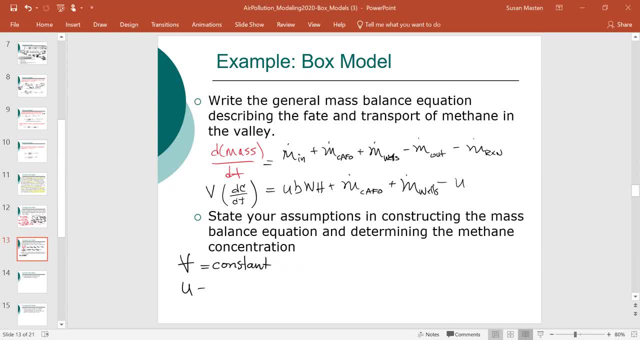 as the same as the wind speed entering. So I'm just gonna write U equals U in, equals U out, So the wind speed doesn't change, It's the same in the cell and leaving the cell. So times my concentration, times my H, and then minus K C. 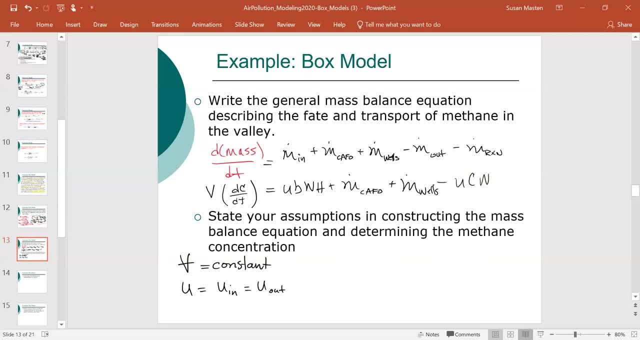 And remember we always use V, So we'll use WH, bright and head. So I've just written in terms of each of those terms. So we've assumed volume is constant, wind speed is constant And it's constant across the cell. 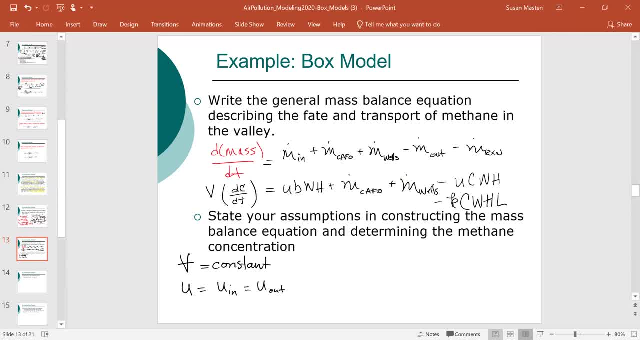 It's also still constant across the cell. It's also constant across the 2024 oxygen cycle, which means school Now copperä. it's also constant in time and space. so it's constant both in time and space. we'll assume that our emissions, emission rate is constant. we're going to assume. 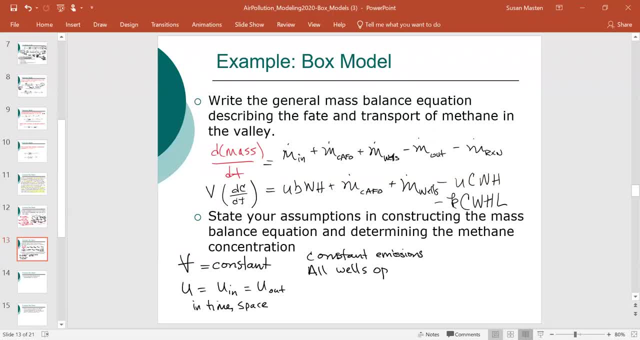 let's assume all the wells are operating. we're going to assume it's a well next systems so that C in the cell it will see out. and we're going to assume that my mixing height is constant over the time studied. basically, my inversion layer isn't lifting any other. 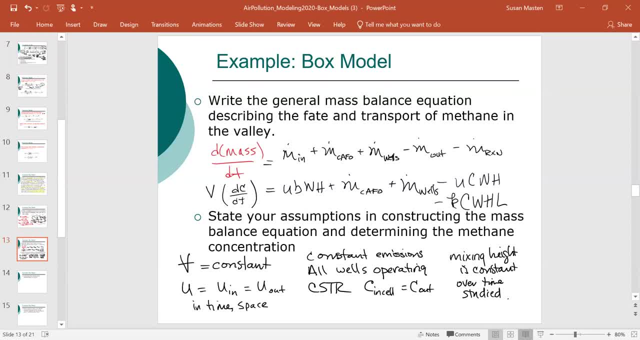 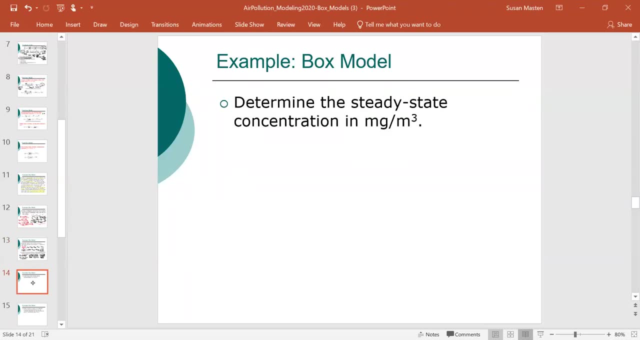 assumptions. we should add here thoughts on assumptions. okay, so the next thing you're asked, I'm asking you to do, is to determine a response that you think is reasonable: the steady-state concentration. So I have steady-state conditions. That means that the change in mass with respect to time is equal to- and here's where I'd wait. 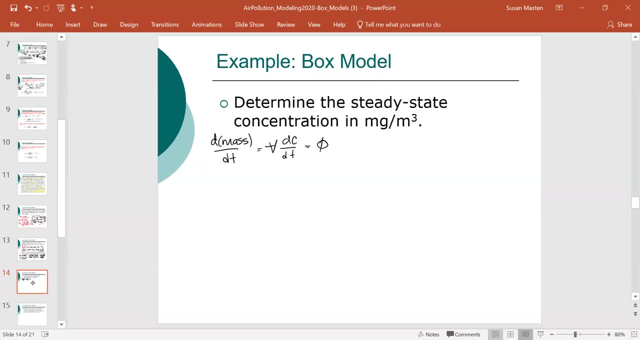 for the answer, but I will just write it zero. And then we have that equation that we just used. So that is equal to 5.1 meters per second. so our wind speed times the concentration, and I'm going to put everything in grams, Remember this. 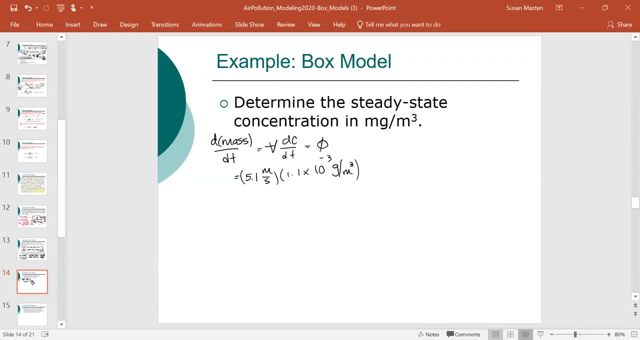 was in milligrams, so I've just converted it to grams per cubic meter. I need to put to convert all of my distances to meters. So now meters cubed, I've got meters, meters, meters and meters cubed. that cancels and I have units of grams per second per source, Plus 15.25. 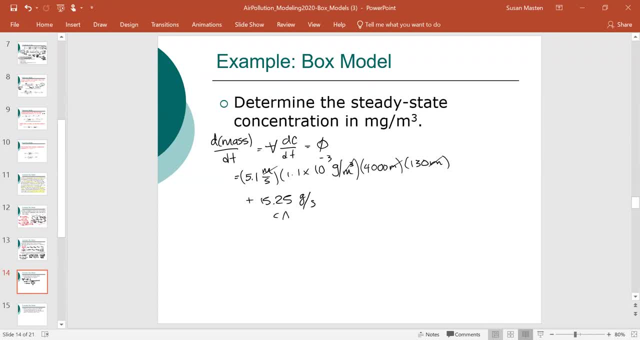 grams per second, that's from my CAFO, plus 15.25 grams per second- that's from my CAFO, plus 35, 3550 grams per second from Mike Wells, minus C times 5.1 meters per. 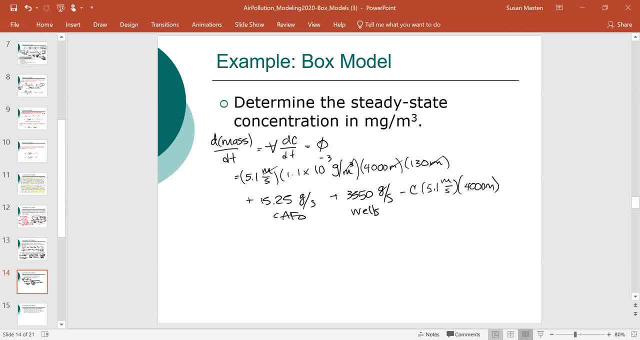 second times 4,000 meters per one cubic. I'm sorry, 4,000 meters times, that was my width and my height. and then, lastly, minus 2.0, 1,, 4 times 10 to the minus 7 inverse seconds time c times 4,000 meters times. 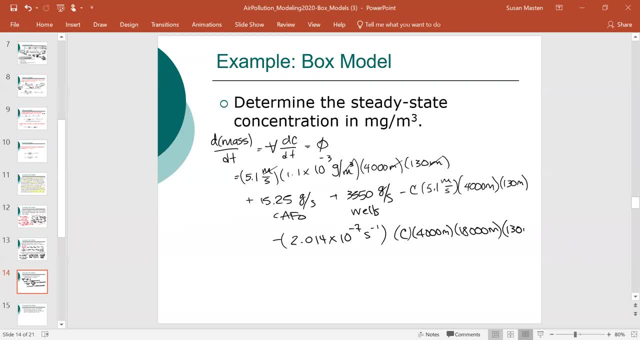 1800 meters times 130 meters- and I can solve for c and c- is equal to 2.0 meters by 10, times 7 inverse seconds, times C, times 1.0 meters. So that's minus 2.0 meters and I'm going to put this in grams: times 5,000 meters, times 6,000 meters: And I can solve for C and C is equal to 2.0 meters times 7, males and Bras, х times C times I, and I'm going to put these into less than 3.. closing up, a bunch more numbers. 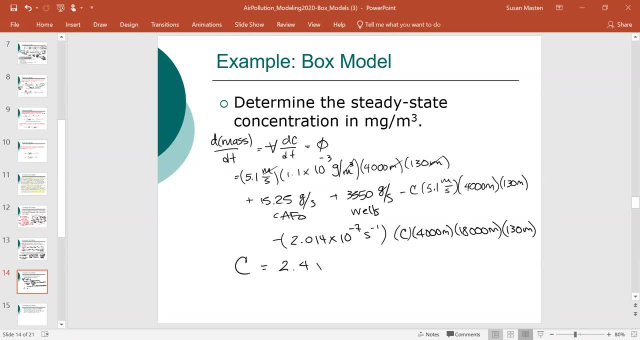 Geassiness and snug teste, and then you just start it over and round groove as I move through time And then you see these little后 equal to 2.4 times 10, to the minus 3 grams per meter cubed, or 2.4 milligrams. 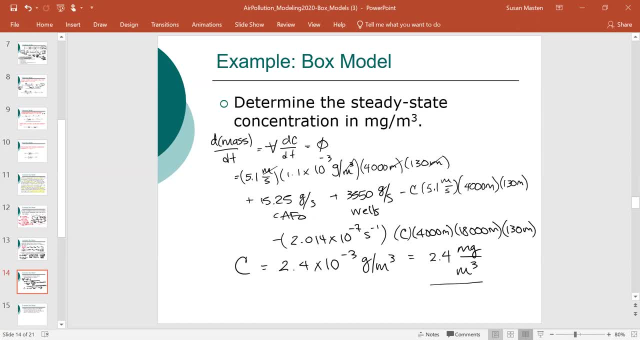 meter cubed. That would be under these operating conditions, with all of the wells operating, with all of the cattle in this cell. This would be I would end up with, at steady state conditions, a concentration of 2.4 milligrams per liter. So it's increased from 1.1 from the previous, from the 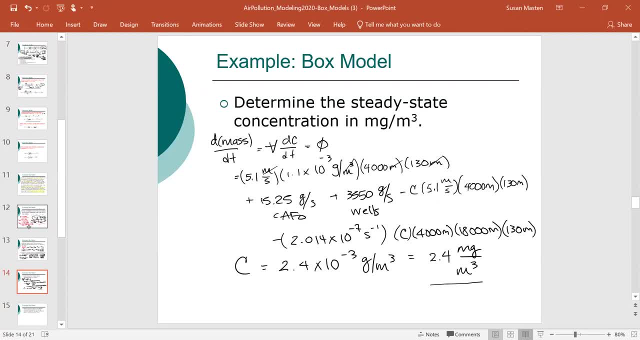 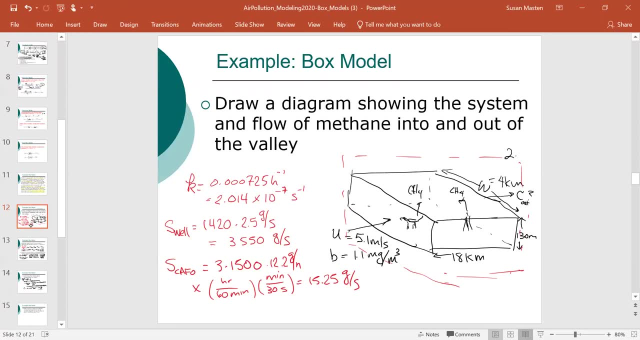 adjacent cell. So if we go back here, remember this was 1.1, and now what is that? Yes, with 2.4 milligrams per liter. But here, if you go right here, you can see leaving is 2.4 milligrams per cubic meter. So that's the concentration leaving. 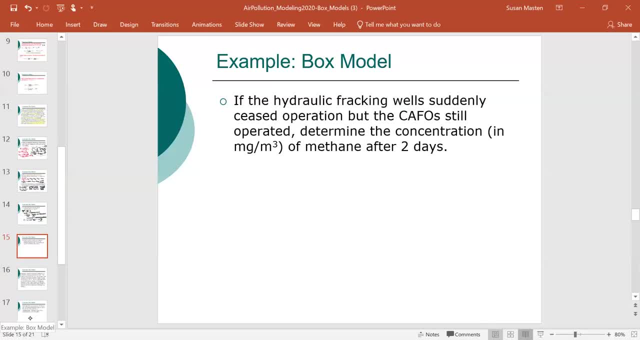 Now what would happen if all of the hydraulic fracking wells suddenly ceased operation? So we've got a condition here We're going to start. We've achieved steady-state conditions, So this is what we start with. For whatever reason, all of the hydraulic fracking wells stop. so we have no wells. We still have the. 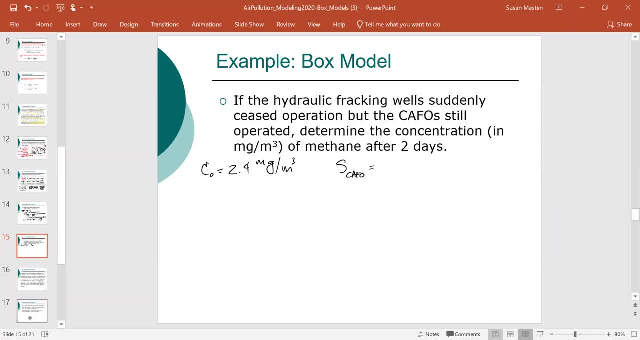 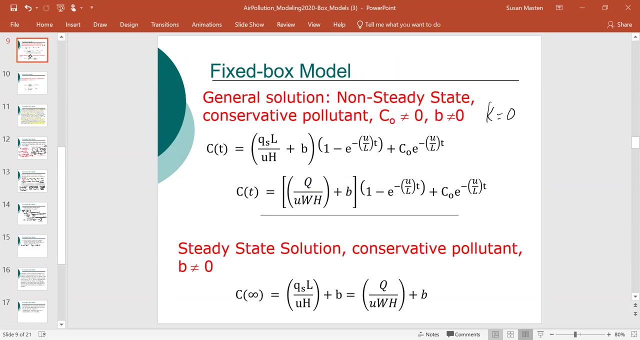 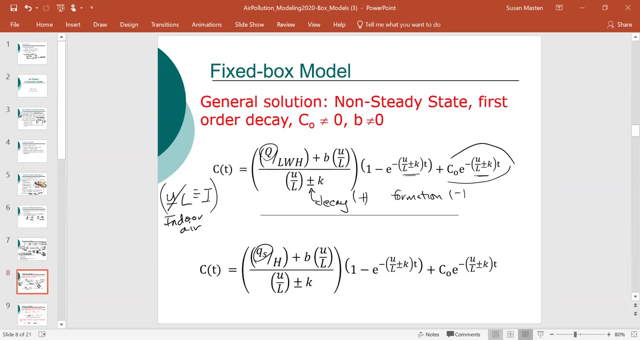 source term for the CAFA. So now this: This is that Q We can go back to. let's look at equations. Okay, what do we have here? Okay, we have. it's not the right one we want. Let's see. Okay, so we have a non-steady-state. 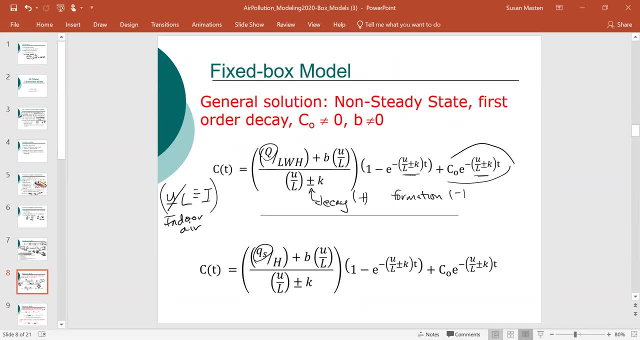 solution And we have first-order decay, We have a C-not term and we have a B term. So this is the equation we're going to use. So we're going to use. So this is now the equation that we will need to use. 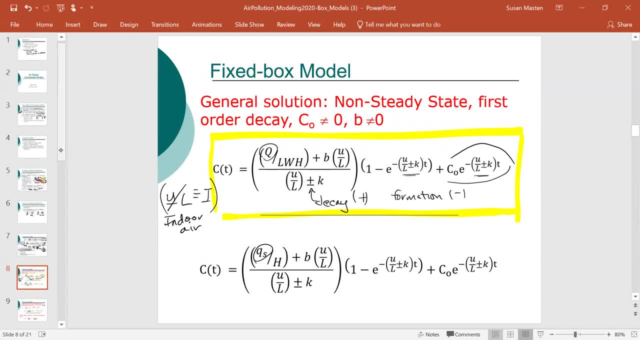 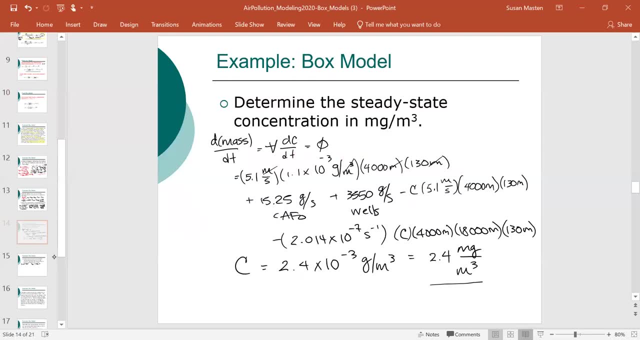 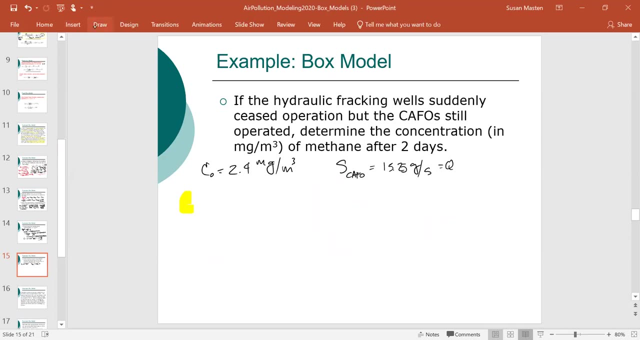 We go back here, okay. so what we want to know is: what is the concentration we're looking at, sorry. so what look? we want the concentration two days after this operation ceases. so we have 15.25 grams per second. we're going to divide that by. 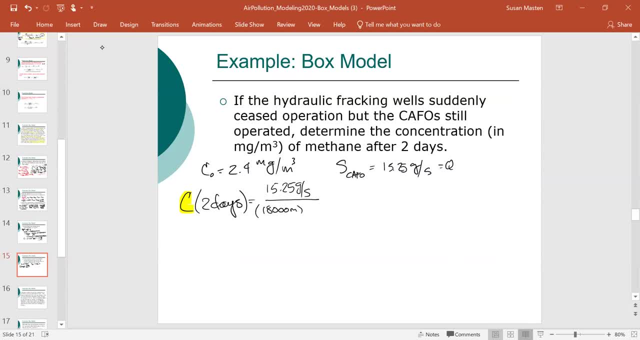 the volume plus 1.1 times 10 to the minus 3 grams per cubic meter- that was the b term- times 5.1 meters per second. so it's u divided by l. we're going to divide that by 5.1 meters per second. 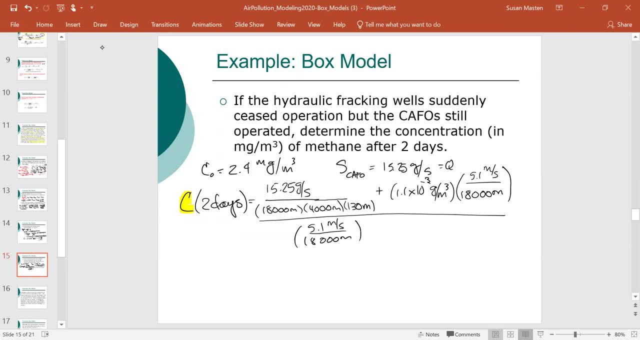 over 1800 meters- again, that's u over l plus k. we're going to multiply that by 1 minus e to the minus 5.1 meters per second. over 1800 meters- again. that's u divided by l plus my rate constant. i need to multiply that by two days. 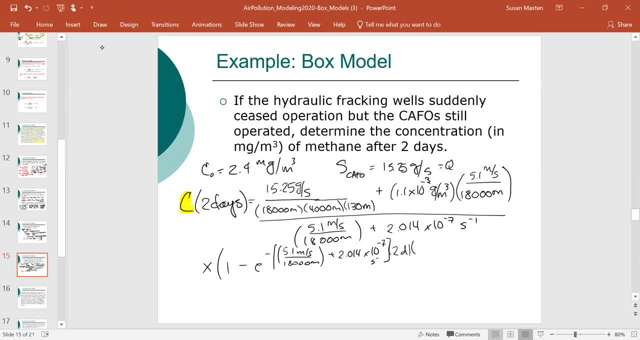 this is in inverse seconds. so we need to multiply by 86 400 seconds per day, plus that last c, sub, not term, and that's e to the minus, and this is again the number of seconds that we need to multiply by two days. exactly the same thing here. 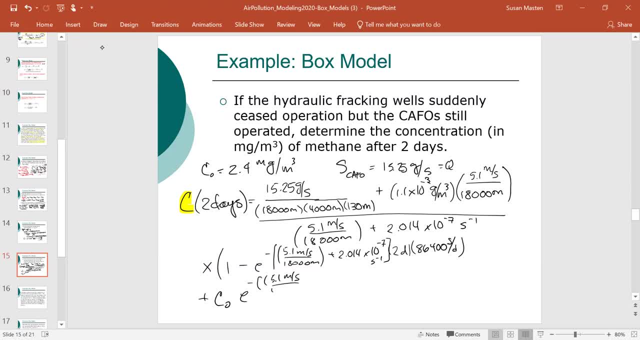 5.1 meters per second. over 1800 meters plus 2.014 times 10. to the minus, seven times two days, 86,400 seconds per day. And lo and behold, we finally do the math and we actually end up with 1.1 times 10. 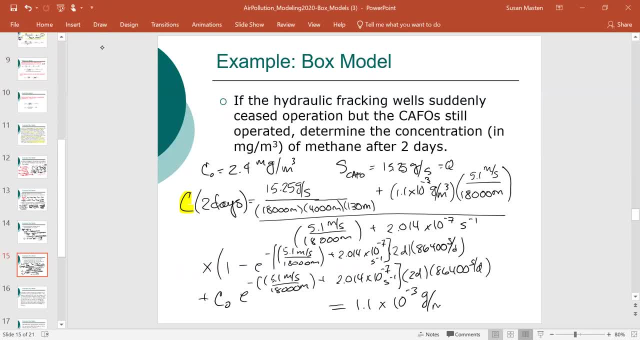 to the minus three grams per cubic meter, or 1.1 milligrams per cubic meter. So the moral of the story is, in this case, with under these conditions, in this size cell, the capos actually don't have any significant contribution to the concentration of methane. 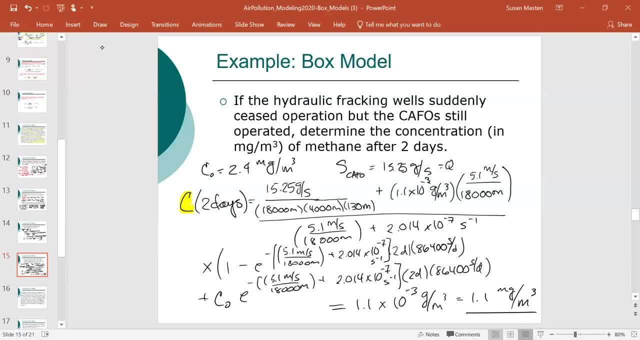 It's entirely the wells that were contributing to their concentrations. That's surprising, really: The wells. the source from the wells was 3,500, roughly 3,500 grams per second, but only 15 from the capos. Questions about that problem. 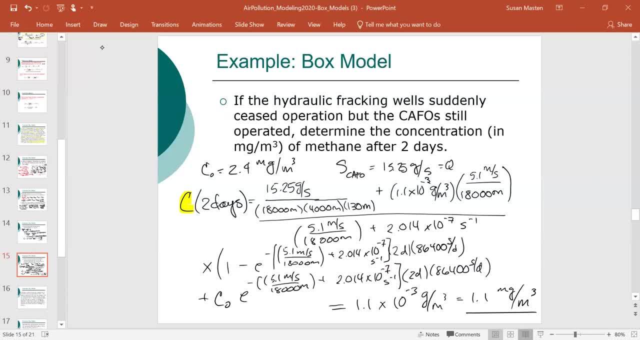 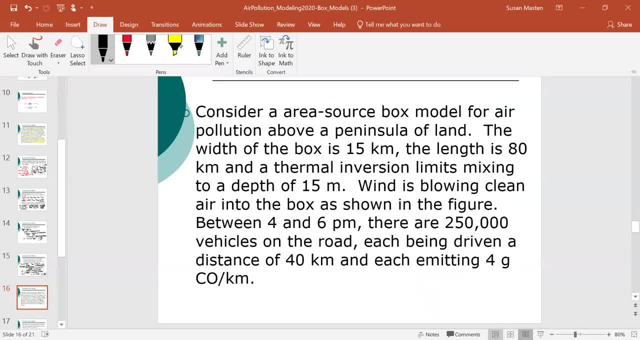 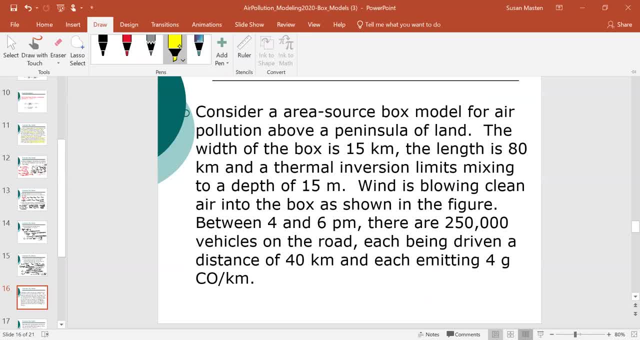 But let's take a look at this one. If you have any questions, feel free to unmute your. you should be able to unmute yourself. Feel free to do so and ask case. we have a similar situation. we have an area source and in this case, we have 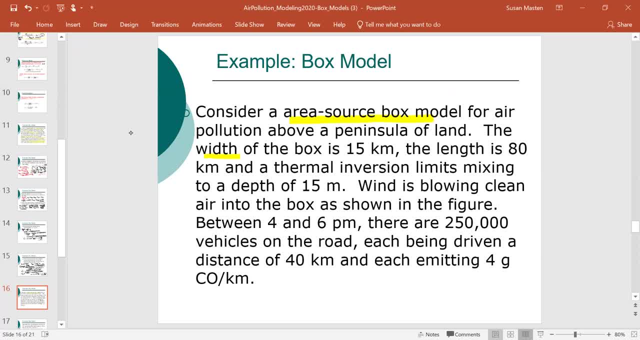 it's going to be cars. so what do we have? we have a width of the box of 15 kilometers. we have a length of 80 kilometers and we have a thermal conversion and it's limiting mixing to a depth of 15 meters. we have wind, that's. 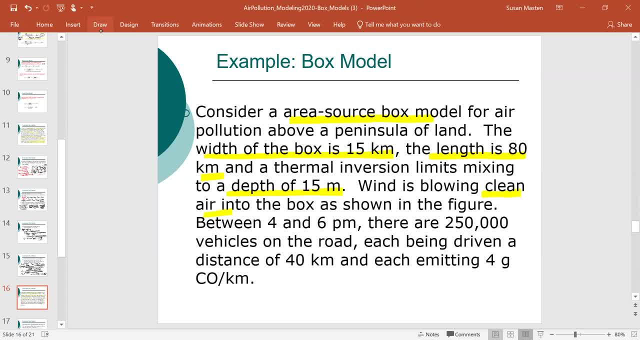 blowing clean air. so in this case B is equal to 0, and between the hours of 4 and 6 pm we have quarter of a million vehicles on the road, and in that two-hour time span they each drive a distance of 40 kilometers and they're emitting four grams of. 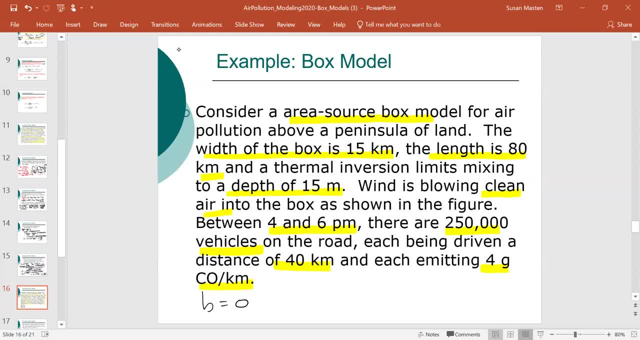 carbon monoxide for each kilometer driven. so let's just before we move on, let's just calculate Q sub S. what do we have? so, Q sub s? we have 2500 cars, each car is driving 40 kilometers And each car is emitting four grams of carbon monoxide per kilometer driven. 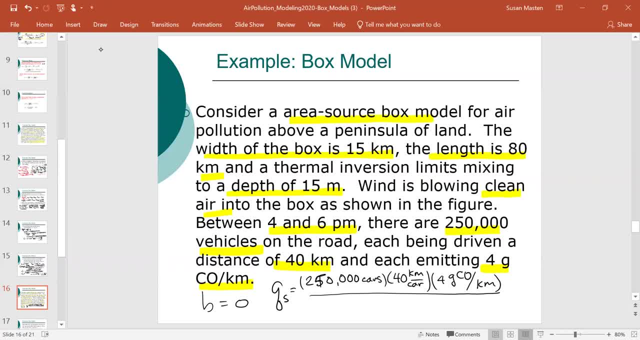 In this case what we're going to do. when we calculate Q sub S, we're calculating per area of the base of my cell, So it's the width times the length, So we have a width. I'm just going to convert this to meters. 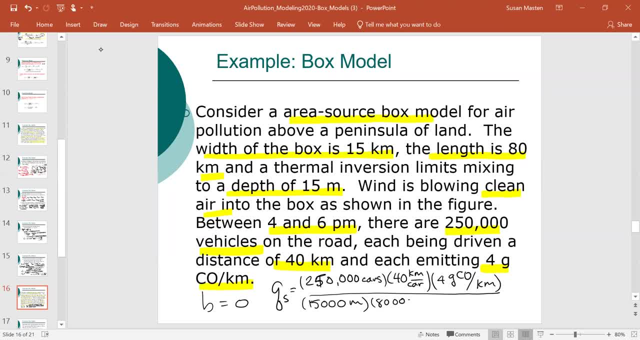 and a length of 80,000 meters And we need a time factor. This is over this two-hour time period And there's 3,600 seconds per hour. So that is equal to 4.6 times 10 to the minus 6 grams per meter squared per second. 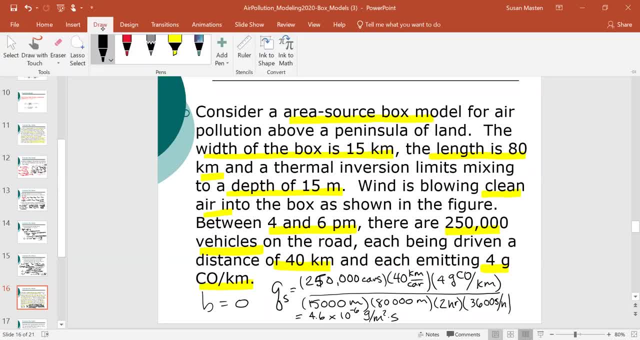 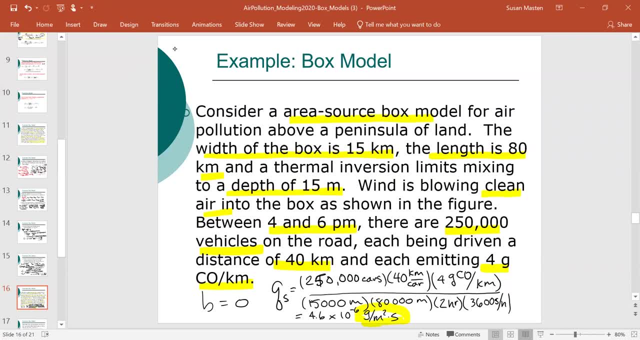 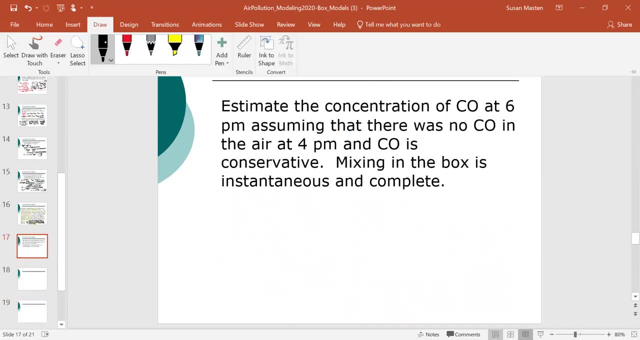 So notice, in this case it's not grams per second, but it's grams per meter squared per second, And what you're asked to do is to estimate the concentration of carbon monoxide at 6 pm, assuming that there's no carbon monoxide in the air. 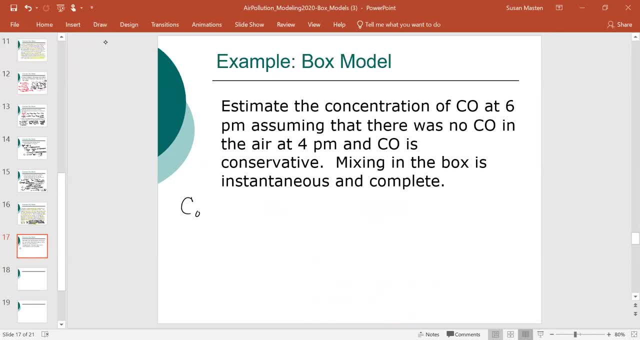 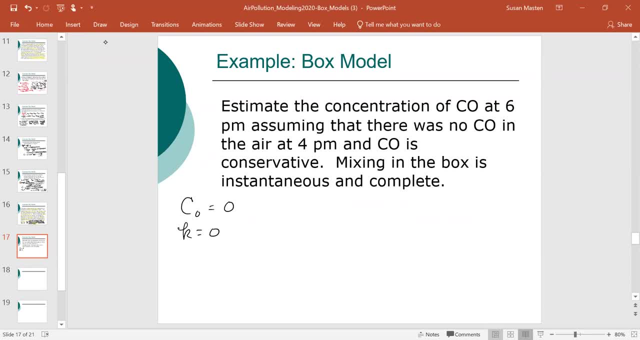 K is equal to zero And we also said that B is equal to zero And we want the concentration at two hours later. So we start at 4 pm. so we're starting at 4.. We're asked: what is the concentration at 6 pm? 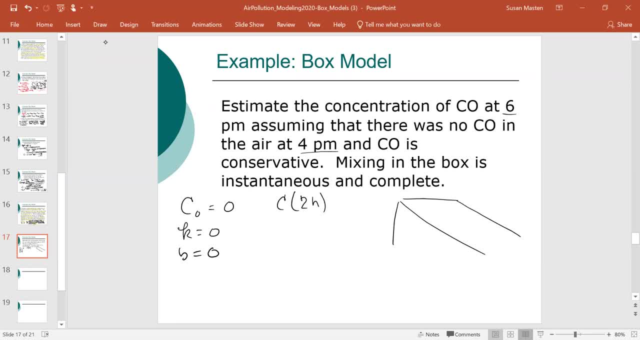 So again, we're going to do this. Here's my box model. I have wind in this direction. It is 0.5 meters per second. The height we said was 15 meters, The length was 80 kilometers. 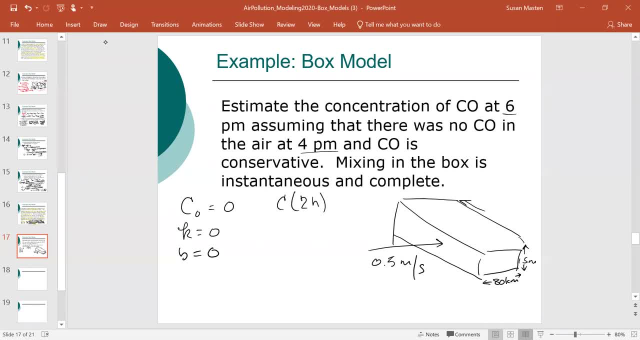 And the width is 15 kilometers, And so that's the conditions we're looking at, And we're going to assume that mixing is instantaneous and complete. So the equation that we can use for this- and these are just from the equations that I gave you before- 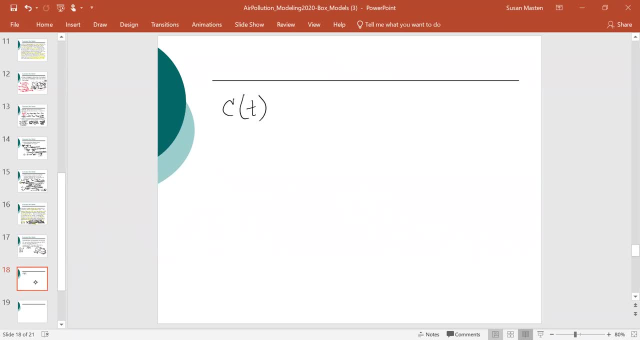 is. CT is equal to Q sub S times the source of carbon dioxide, And we have to do this manually, And then we have to do that manually, And then we have to do that manually: L over U H, 1 minus E to the minus U over L T, And you should be able to go back and look at. 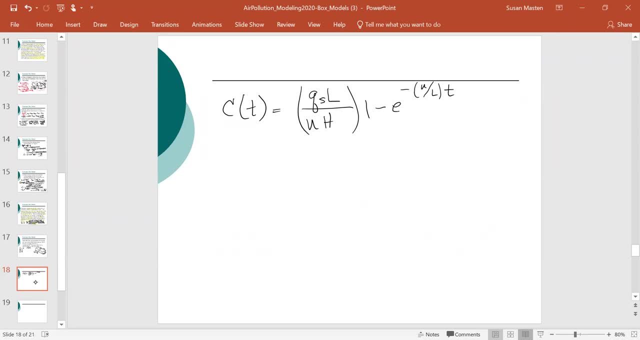 the most general form and be able to derive this equation- And this is 4.6 times 10- to the minus 6 grams of carbon monoxide per second per meter squared. per meter squared times the length, which is 80,000 meters divided by 0.5 meters per second, is our wind speed times the height. 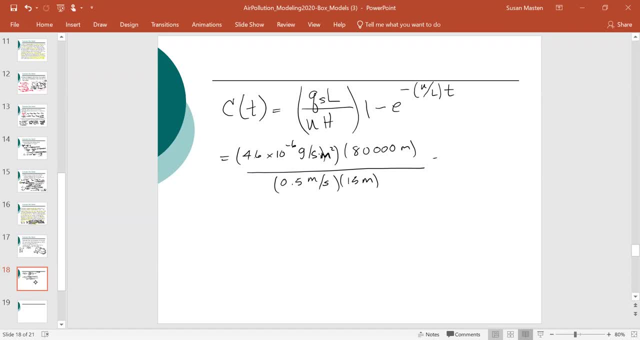 which in this case is 15 meters, And that is equal to 2 milligrams per cubic meter. So that would be the concentration in this cell that I've defined. with quarter of a million cars on the road driving within those two hours, We're. 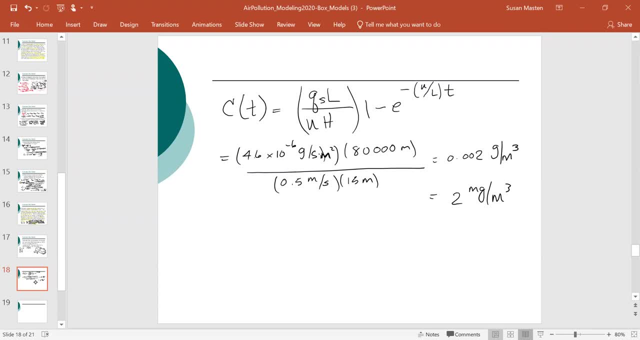 assuming that it's constant within the two hours, Okay. So just thinking back to we haven't mentioned, So we had. we said it was 40 kilometers as per two hours. So we're assuming that they're driving the whole two hours, Okay, Or on average, they're driving the whole two hours. Same sets of. 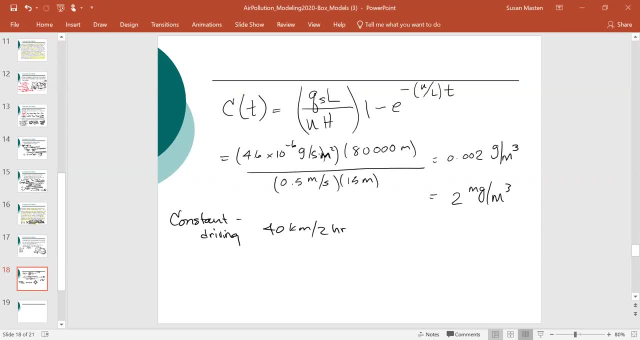 assumptions that we had before in terms of the constant mixing height, constant volume et cetera. And if you just kind of give standard, the one hour standard for carbon monoxide is 35 parts per million, which is 40 milligrams per cubic meter at 25 degrees C and one atmosphere. So this is well below. 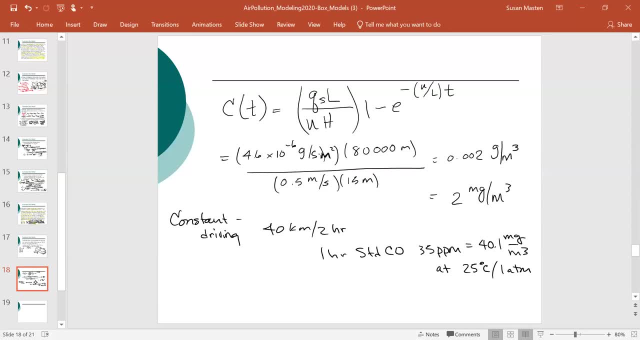 the one hour standard for carbon monoxide. So any questions about what we've done so far. Any questions about what we've done so far, Any questions about what we've done so far. My advice is take a look at the. I mean, you've got the meteorology homework, but if you have time, 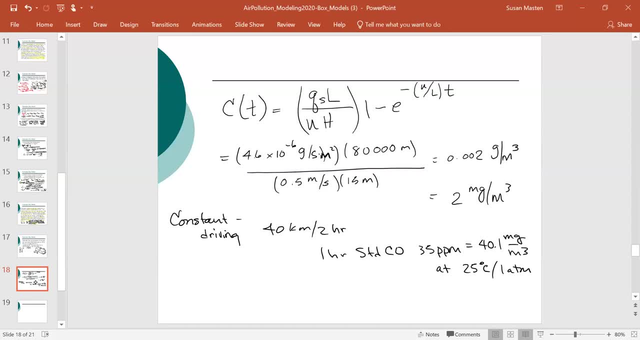 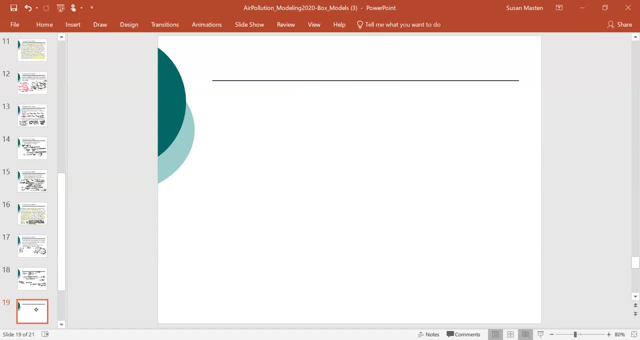 I think it's the best way to ask a question. Okay, the homework. you do have one problem where basically, what it is is you've got a series of cells and i'm just going to draw them separately just to make it a little easier to think about. 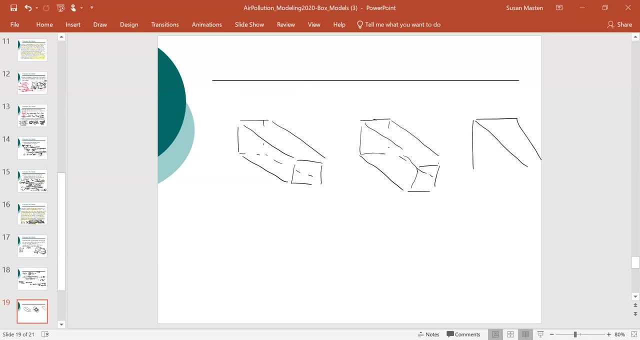 so there is one problem like this: okay, and basically you have air coming in here, so you've got b and i'm going to call that b1, and then you've got c1 leaving. that is going to become b2, and then you have c2 here. that it. 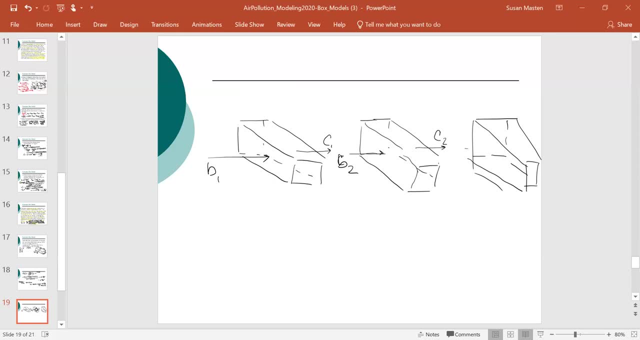 becomes b3, and then you've got c2, and then you've got c1, and then you've got c2, and then you've got c3, and then you have c3. so basically what you have is you have a series of cells, so an area that you've divided up into three cells, and you're looking at each of them. 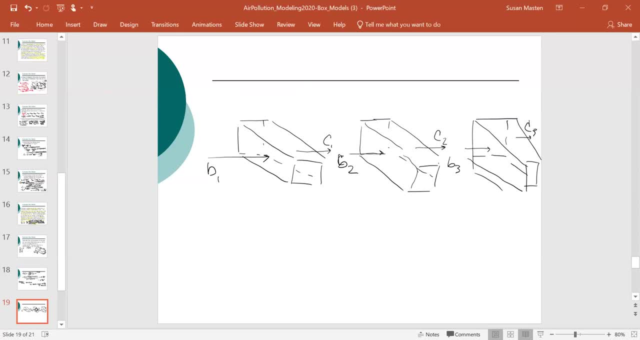 sequentially. so in order to solve that problem, you'll need to divide up that problem to, as i said, three different cells and solve it that way. any other questions? i will add a participation question. um, this afternoon, um, the participation question is going to be the math. um, just to state one challenge that you've experienced over the last week and 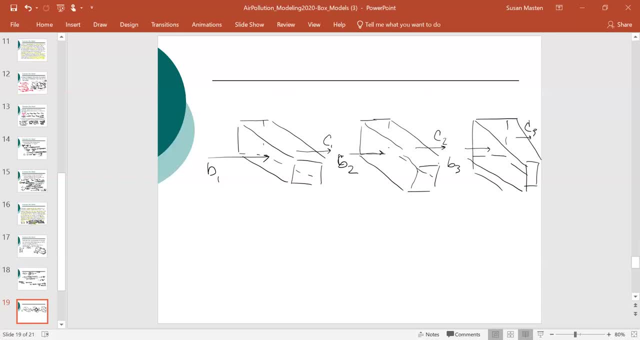 one success. if you don't want to tell me that, you can always tell me just anything. you still get the participation points, but we're going to try and get to the next one. so i'm going to get you to do is think about kind of what successes. 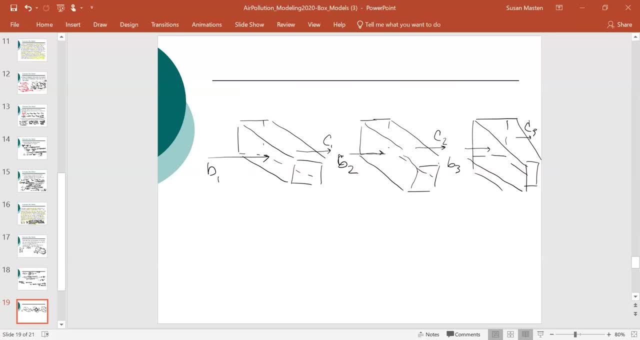 did we achieve over this last week? it's very different time, but hopefully maybe they're minor, but hopefully we've all achieved some successes over this last week. so we'll end there, since i don't have any questions, and i will meet with all of you on monday. then 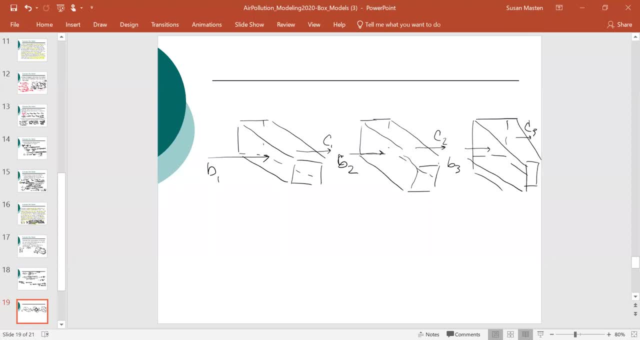 and if you, as i mentioned, if you have questions on doing the homework, just let me know and we can arrange a time to meet. uh professor, yes, i've actually had a question about that car problem. so you wrote out like the ct equals qsl over the uh, and then like what happened with that e term, though, 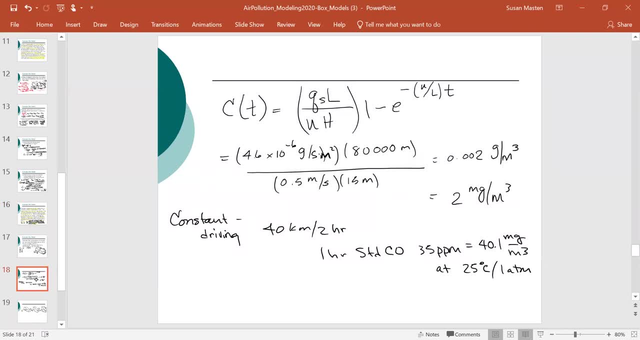 okay, the e term here. yeah, you're right, i didn't write it out. i'm sorry, thank you. one minus e to the minus. thank you for doing that mentioning. i just lost the page um, so this would become u, um, what was it? 0.5 meters per second over.